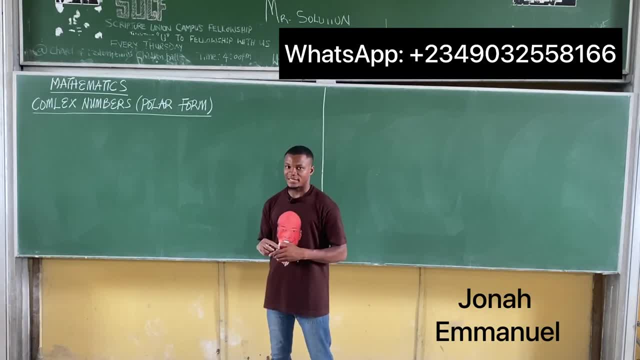 of this video and I'll provide a link to our previous class on complex numbers. But let's dive right into this. So, please, if you missed our previous class on complex number, do well to watch it. So let's get started. So let's watch that class first before watching this one here, so that it will aid your understanding. 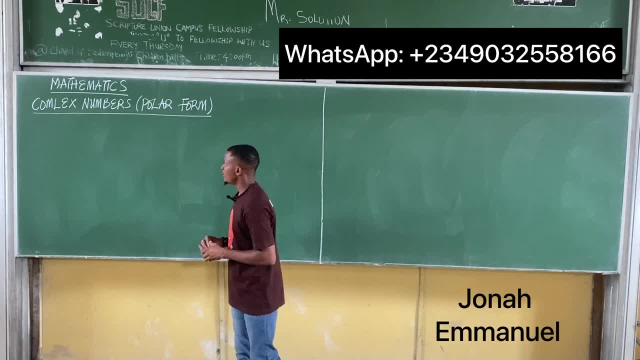 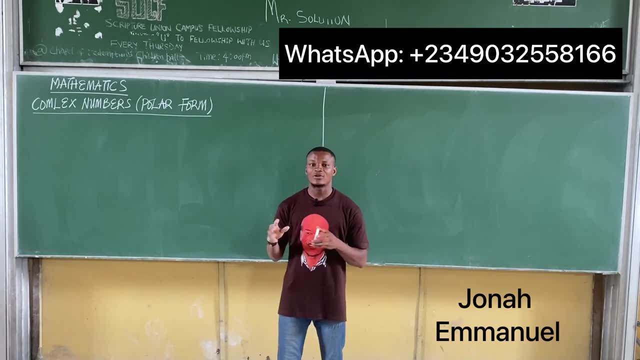 All right. having said so, let's look at complex numbers in polar forms. Specifically, we'll be looking at how to multiply and divide complex numbers in their polar form. The idea of this is that it will help us to understand some certain concepts in Agand diagram, which will be treated. 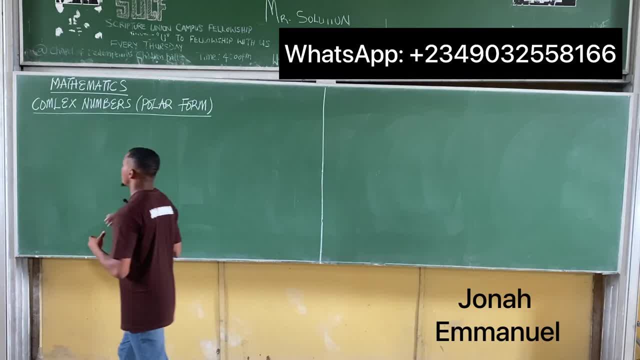 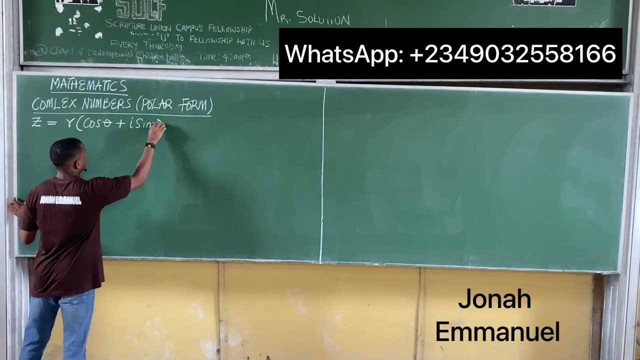 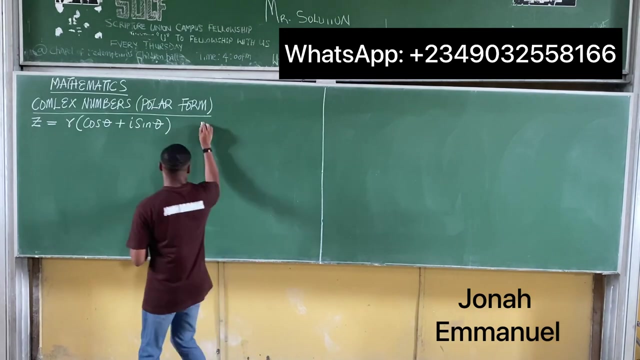 much more later. So for this, first let's recall what we said. We said in, in polar form, that a complex number, z is equal to r into cos theta plus i sine theta. When we said r is called the modulus or the magnitude, and we said so- we said r is called the modulus. 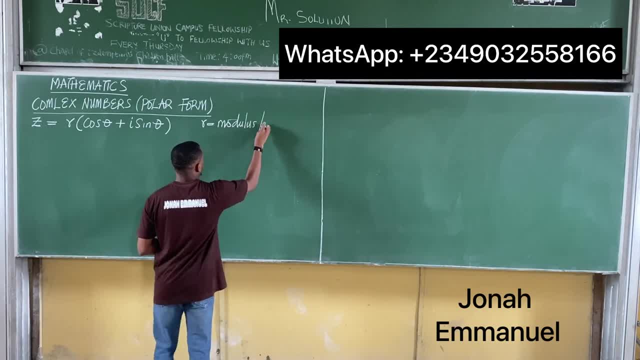 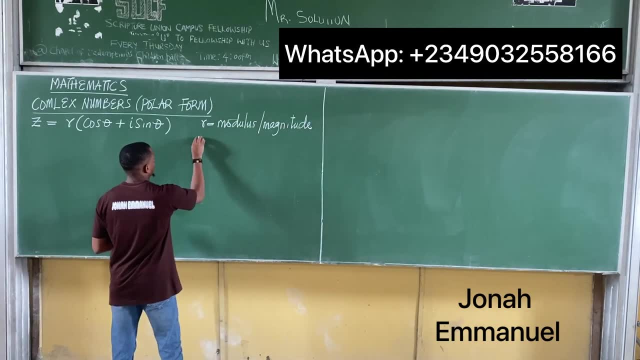 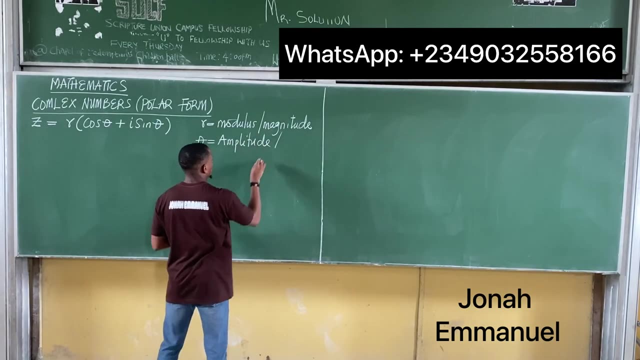 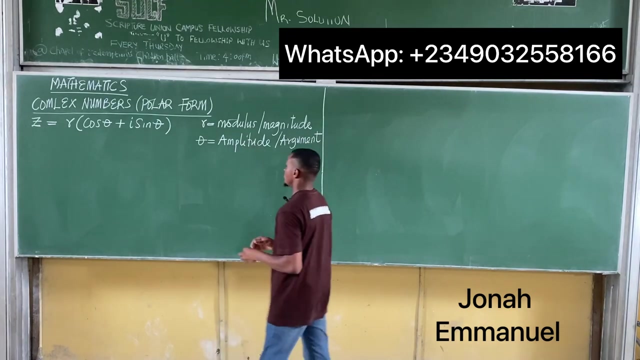 of the complex number said modulus, or the magnitude of the complex number, and we said theta is called the amplitude. Now another name for amplitude is also called the argument. Another name for amplitude is argument. So theta is also called the amplitude or the argument, which is simply the angle there. All right, in our last class I didn't, I didn't mention that. 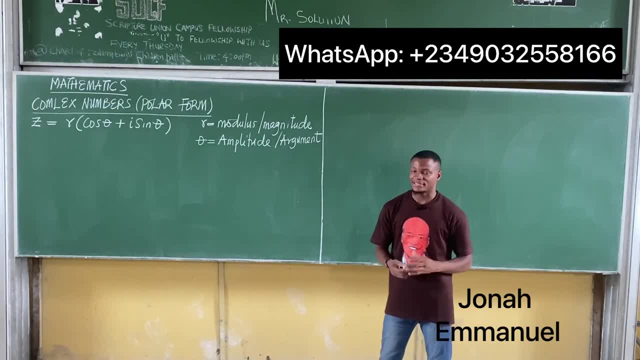 theta is called argument. so you can just note it for this class that theta is also called argument. All right, let's look at something. Let's look at how to multiply and divide complex numbers in. so let's look at something. Let's say we're given a complex number. Let's say we're given two complex 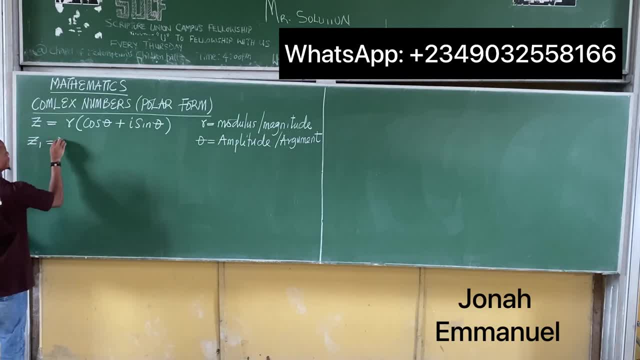 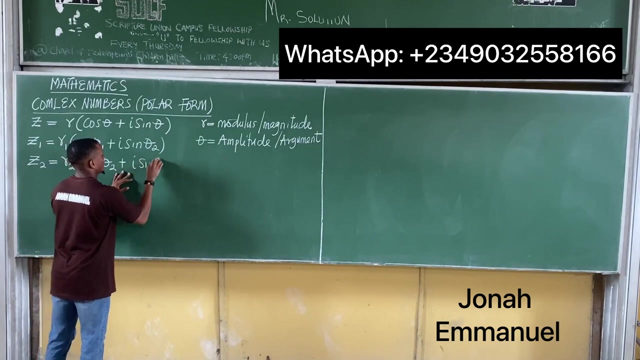 number. The first one is z1 being equal to r1 cos theta 1 plus i sine theta 2.. So here's my first complex number and the second complex number, z2, being equal to r2 into cos theta 2 plus i sine theta 2.. So I have these two complex numbers, If I were to find their products: z1. 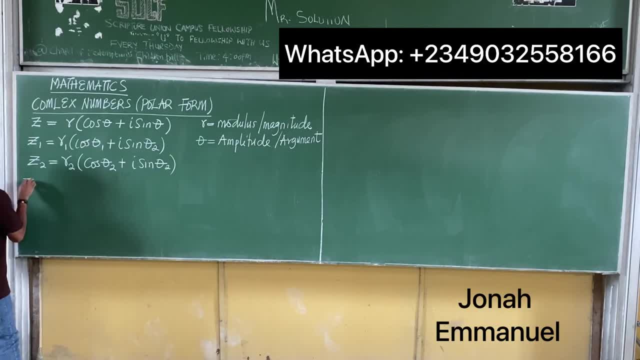 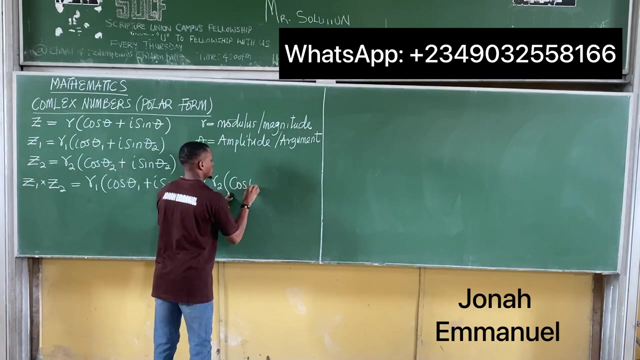 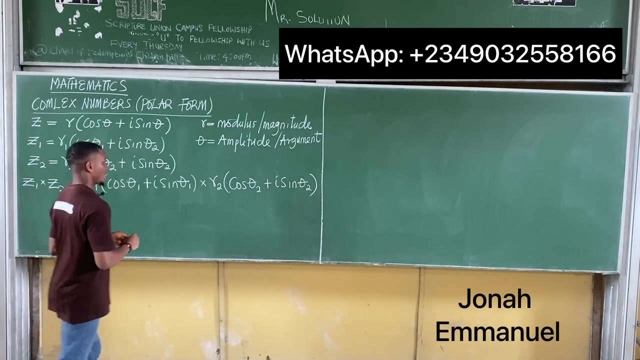 times z2. so I'll have that z1 multiplying z2, or simply z1. z2 will be equal to this. multiplying this, that'll be r1 into cos theta 1 plus i sine theta 1. multiplying that craks r2 into cos theta 2 plus i sine theta 2.. So I have this. so if I multiply this, 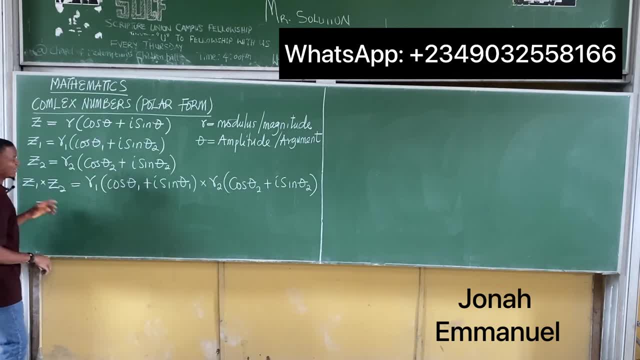 what do I get? This is equal. to know this first, I'll be having r1 times r2. that becomes r1- r2, so r1- r2. so I'm done multiplying this once. yeah, That is the modulus. Next, I'l multiply the terms in brackets. So my first term in the first brackets, that's quotidien. 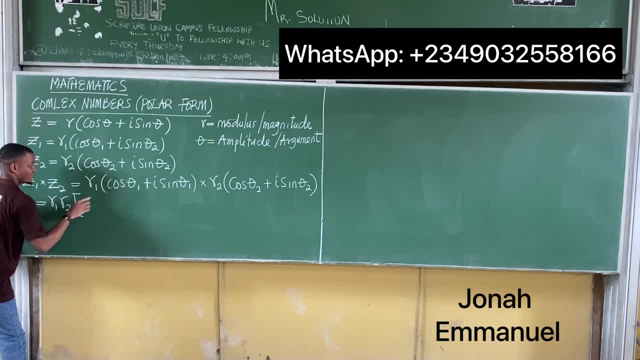 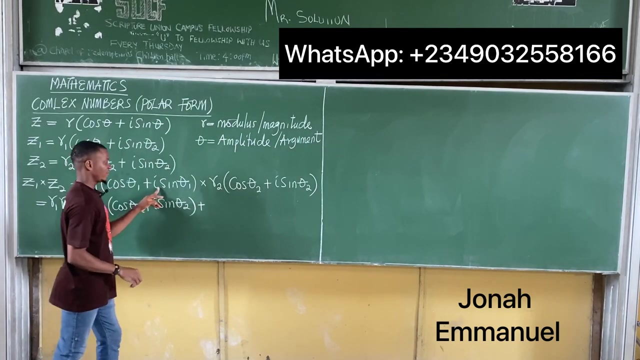 that becomes- this is into the first in the first bracket is cos theta 1 multiplying everything in second bracket. that'll give you cos theta 2 plus i sine theta 2, right. so first in here, multiply everything in second bracket next up plus second term. in first bracket. i sine theta 1 multiply. 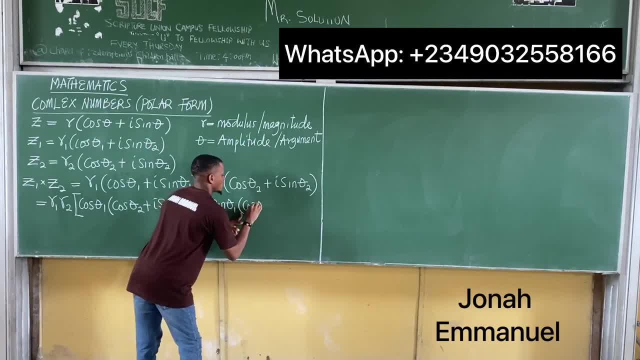 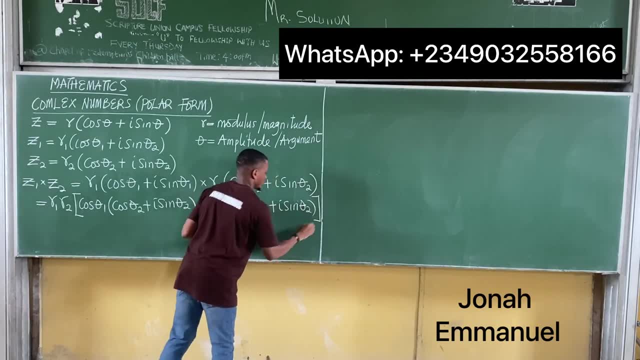 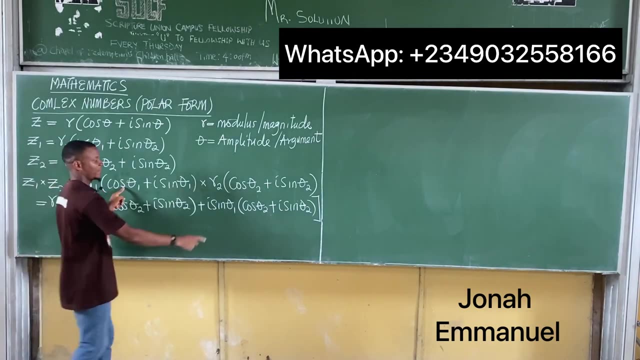 everything in the second bracket, that's cos theta 2 plus i sine theta 2, we have this case all right. so simply multiply the modulus r1, r2- use the first term here, cos theta 1. multiply everything here. next up, use the second term here: multiply everything here. what i want to say this: 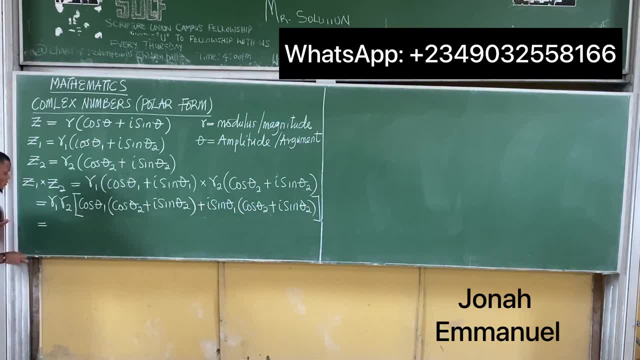 is equal to um, so this is equal, so that's equal to this one. here you r1, r2 all into cos theta 1 times cos theta 2 gives you cos theta 1, cos theta 2 plus cos theta 1. multiplying i sine theta 2 gives you just an i here. so i into this. 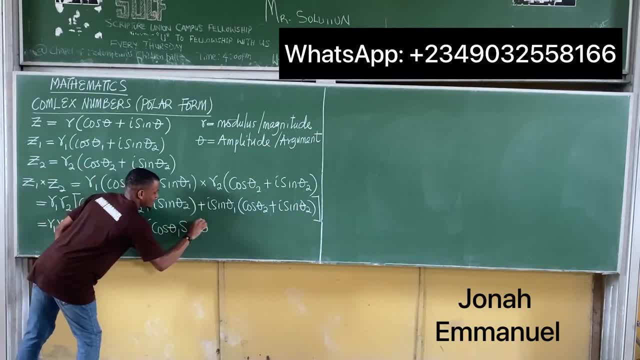 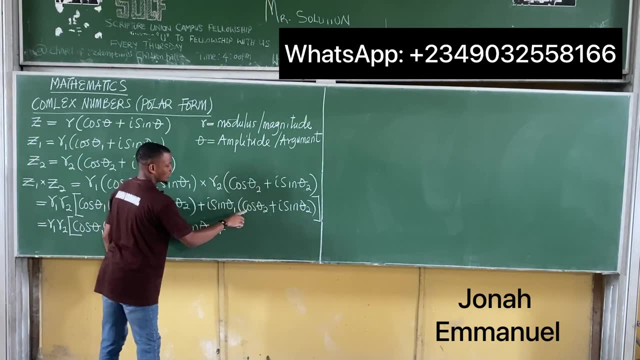 cos theta 1, sine theta 2. okay, use this to expand this. so plus i sine theta 1, cos theta 2, so my i first. so i want to take cos before sine. um is the same thing whichever way, so you can choose to take sine before cos, the same thing. so cos theta 2. 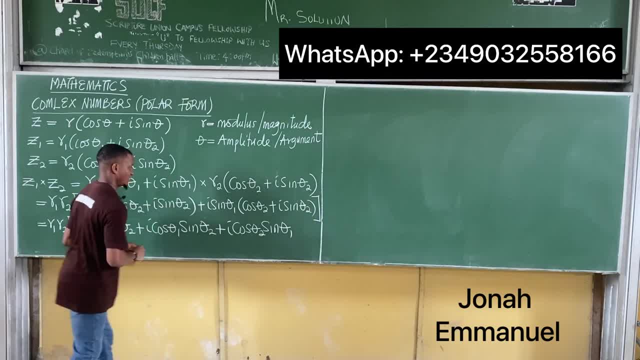 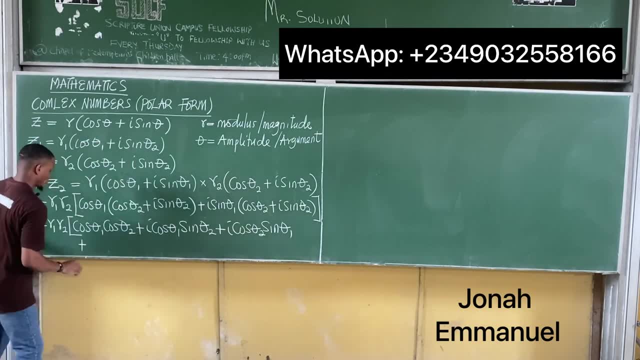 sine theta 1 plus. so plus i now have i times i that gives you i squared, so plus i squared into sine theta 1 multiplying sine theta 2 gives you right, so cos theta 2 cosine is involved sine theta 2 time, sine theta 1 love. 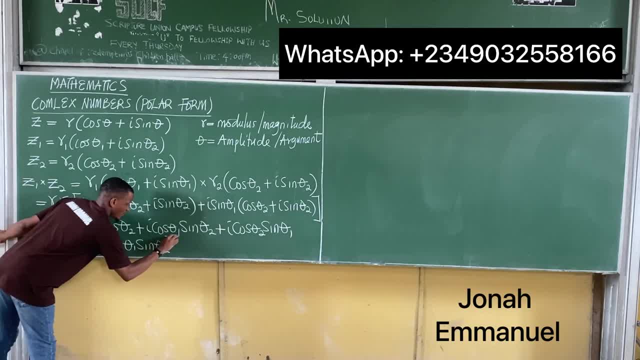 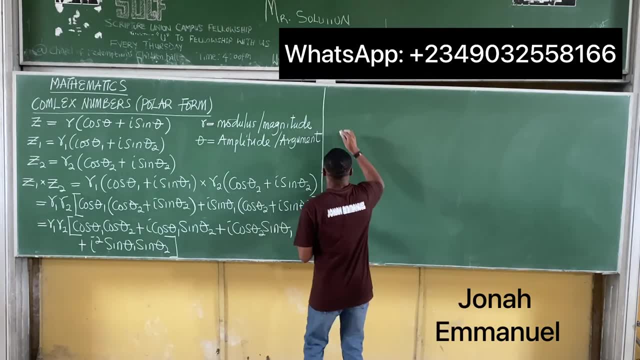 so i have this one here, all right. so this is my case. on expansion next up, we'll try to simplify this. so if i try to simplify this, i have r1, so that's equal is equal to what do I get? R1, R2. 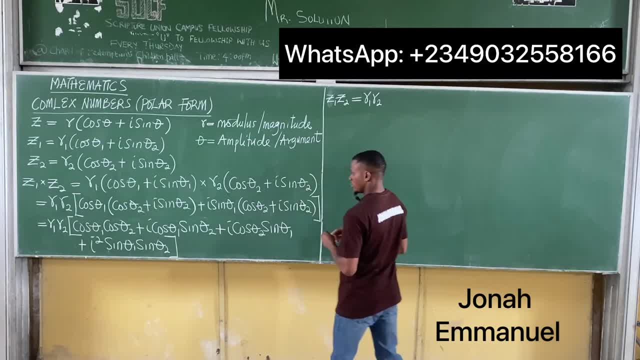 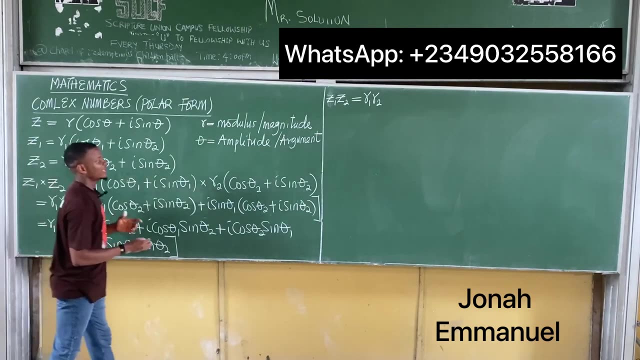 so I have R1 R2 into. for the case of time, I will simplify everything here now. what I mean is this: from here, if I multiply, I squared. I know that I squared gives me minus 1 because we said so in a previous class. we said: I is equal to. 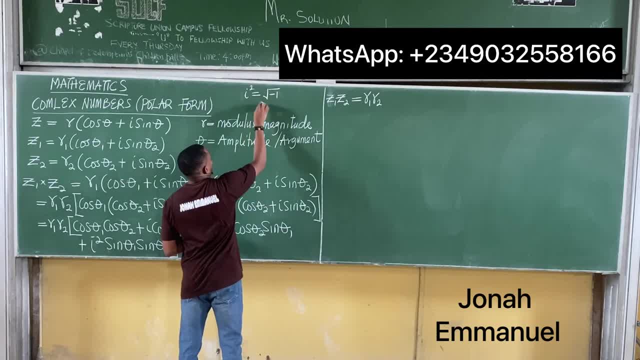 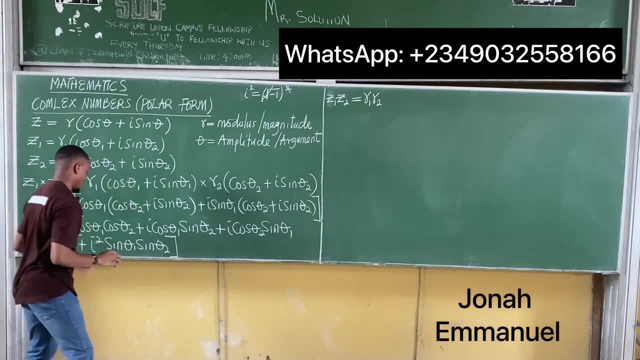 square root of minus 1, so if I square, I becomes all of this squared, such that the square and the square will cancel square root. I have minus 1, hence this one here will give me a value of minus 1, so I have minus 1. 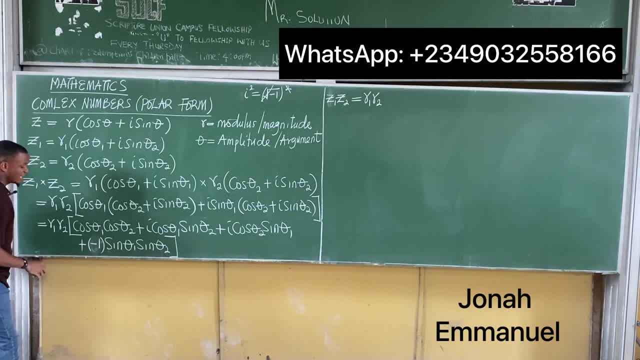 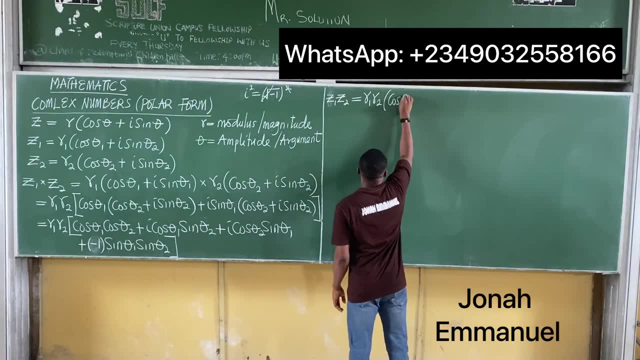 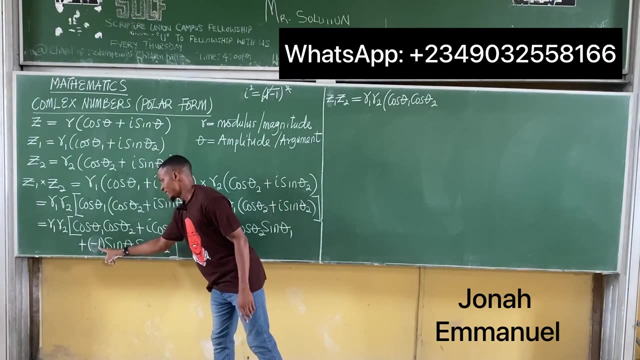 here, multiplying all of this such that if they multiply I'll be having cos theta 1, cos theta 2, so into cos theta 1, cos theta 2, into plus times. minus 1 is minus 1 times. this is itself, so that becomes minus. 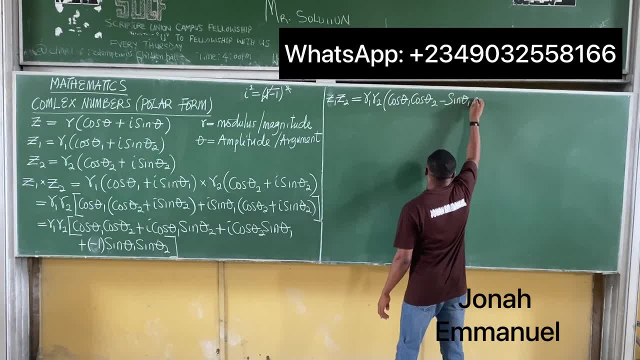 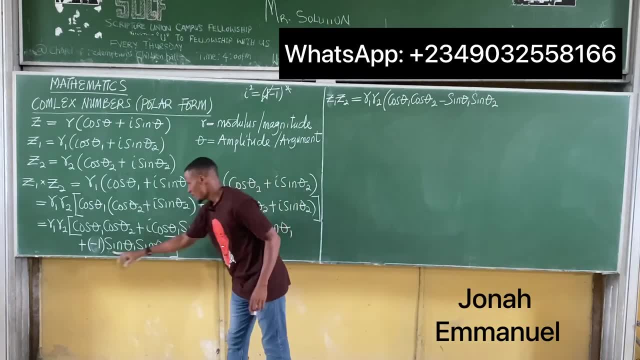 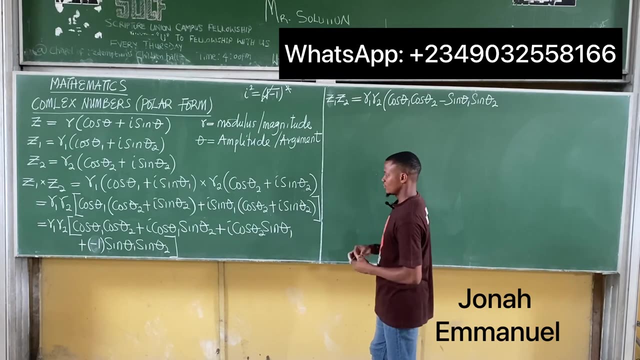 that becomes minus sin theta 1, sin theta 2,. alright, so I have this. alright, so minus 1 times this gives you minus theta 1, or minus sin theta 1 minus sin theta 2, now take the imaginary parts. that's the I's. so I have this one. 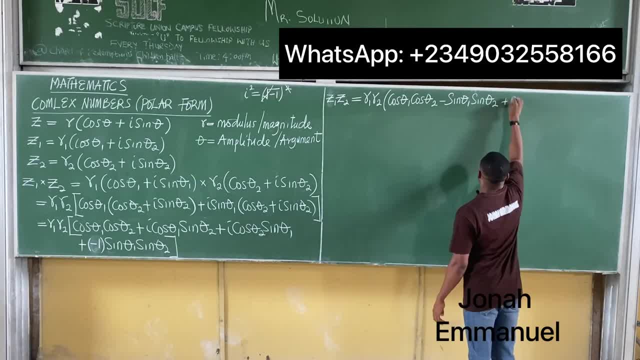 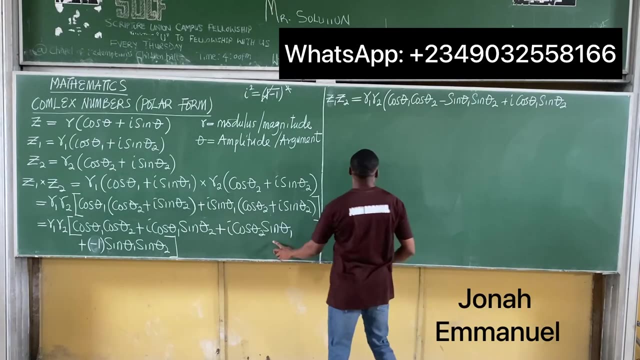 here. so plus I, so plus I into the first one. here is cos theta 1, sin theta 2. that's cos theta 1, sin theta 2, and then a final I, so plus I, so plus I into cos theta 2, sin. 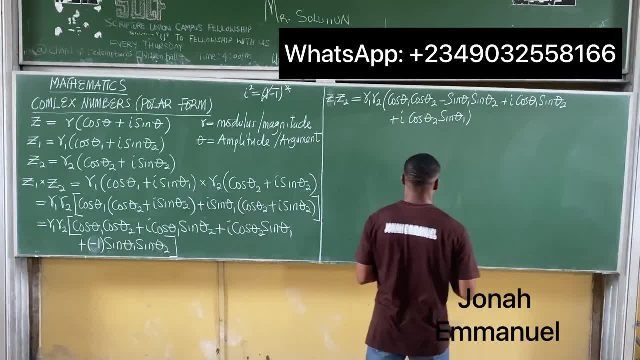 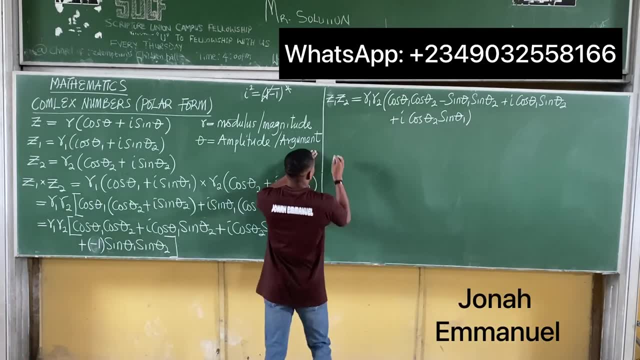 theta 1, so we have this one here, alright. so if we have this case here, we can choose to factorize the I's. ok, let's factorize the I's. we'll have that: z1, z2,, z1, z2. 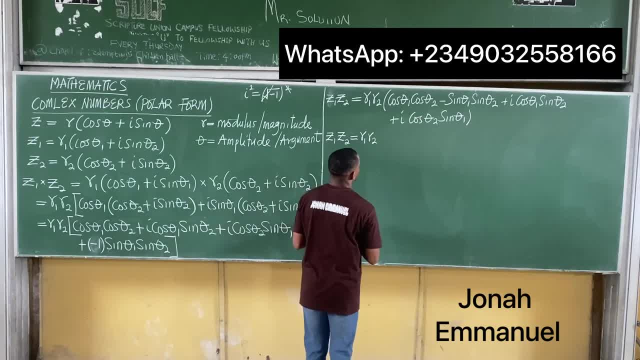 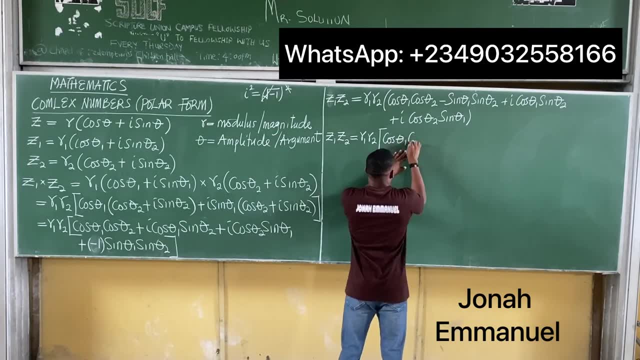 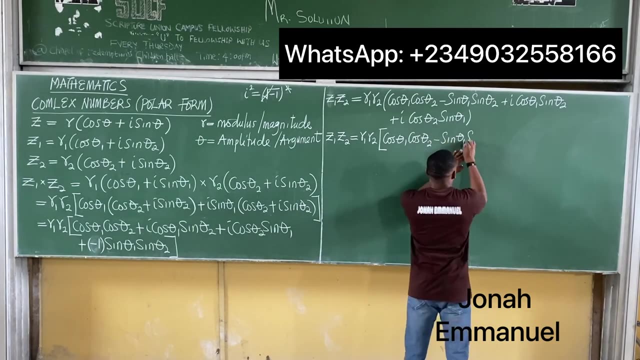 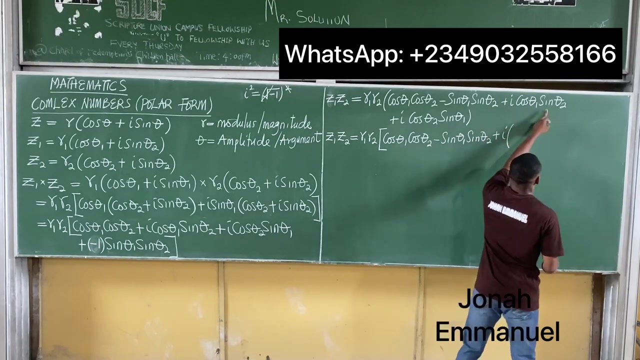 is equal to r1, r2 into. I'm having this one here as cos theta 1, cos theta 2 minus sin theta 1, sin theta 2 plus I. into factorize the I's. I'm having this as plus cos theta 1, sin theta 2.. 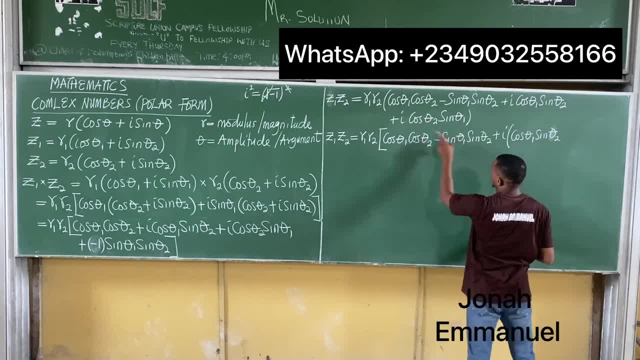 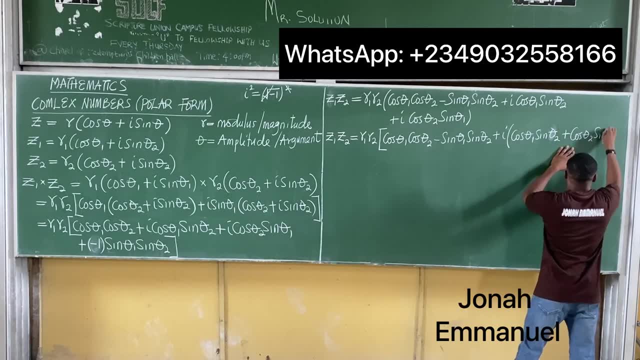 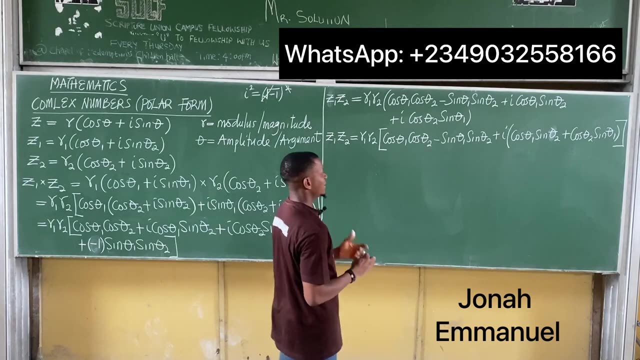 I'm going to write this properly, And then this one here, plus cos theta 2, cos theta 2, sin theta 1.. So I have this when I simplify, So I have this one here. All right, so we are now at this point, after expanding this one here. 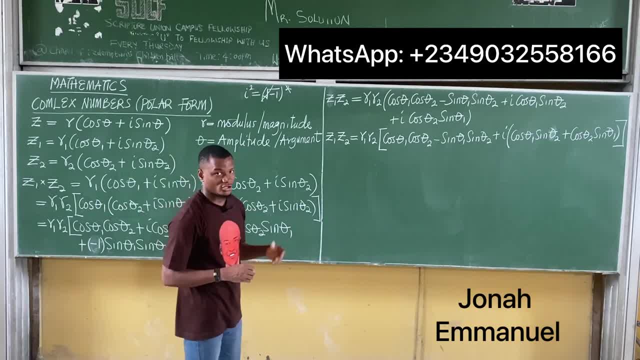 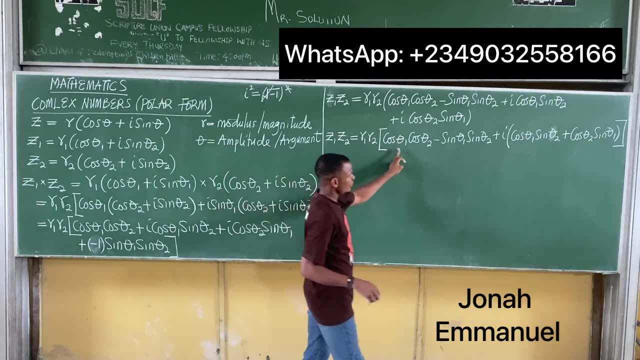 that's multiplying two complex numbers in third form or in polar form. please, two complex numbers in polar form. My next task would be: from this I can see a trigonometric identity. Remember that from trig functions we said cos. that's how we cos. 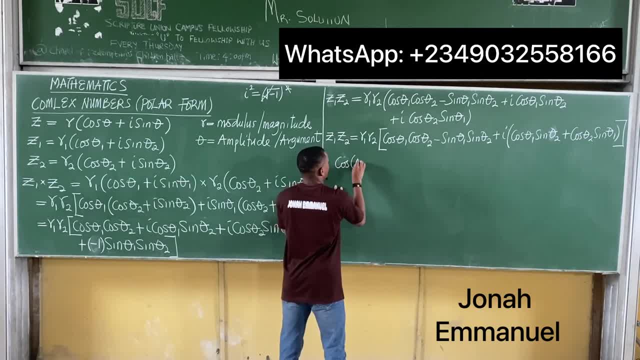 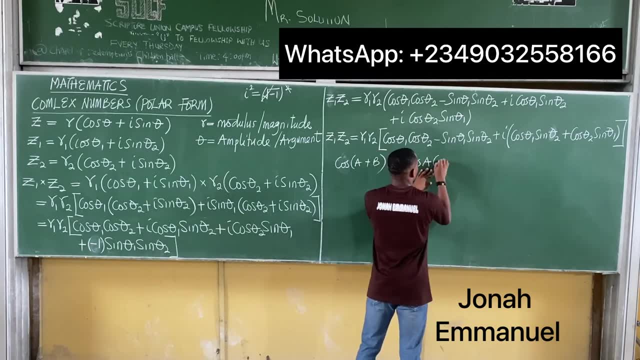 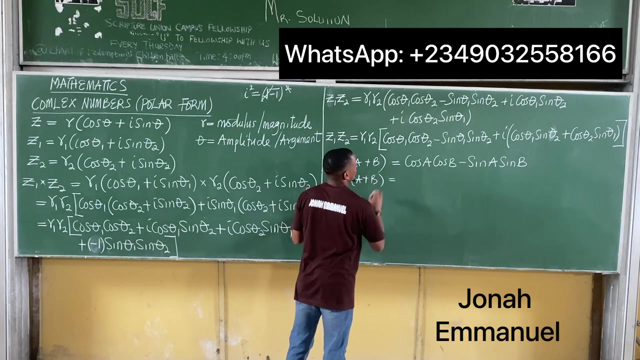 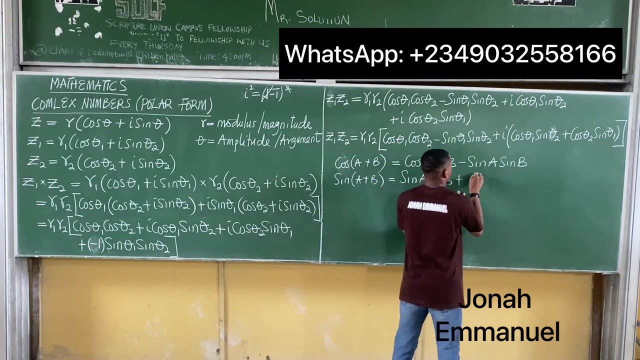 we said: cos cos a plus b- this is a trigonometric identity- is equal to cos a cos b. This is a trigonometric identity. We also have that sin a plus b is equal to sin a cos b plus cos a sin b. 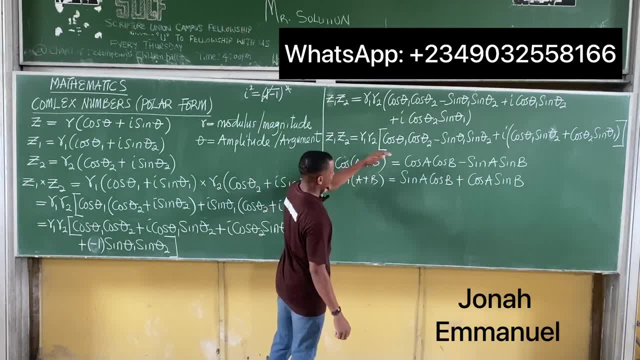 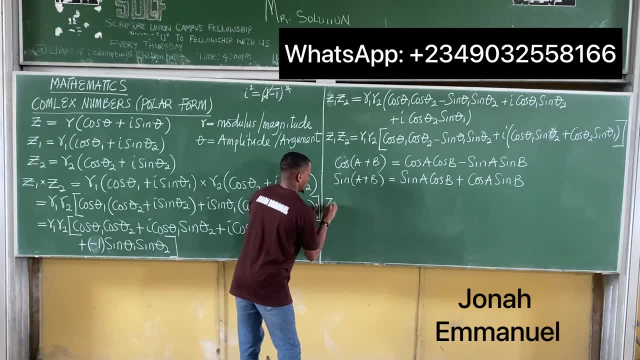 All right. so with these two ideas, now we can write this multiplication, or we can write this multiplication, or we can write this multiplication or this product in this form, such that I'll have that z1,, z1,, z2. 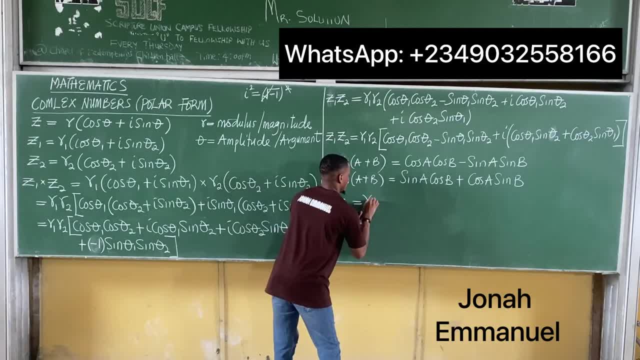 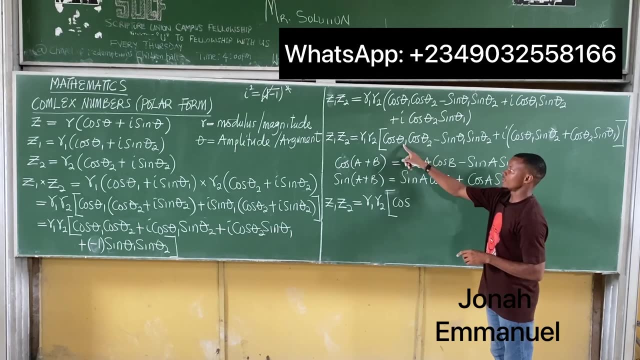 is equal to r1, r2,, that's r1, r2, into, into I have cos. Now observe that if I have, if this was a and b, if theta 1 was a or I've had cos a, theta 2 is b or I've had cos b. 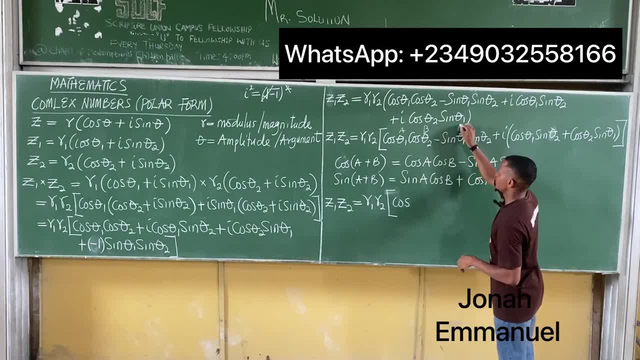 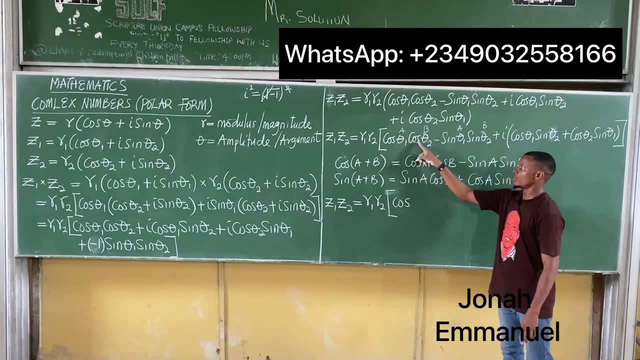 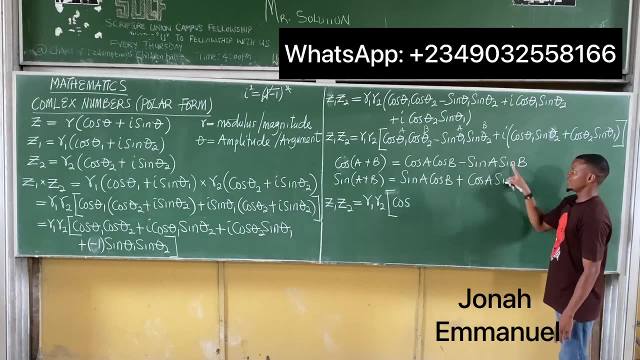 minus. we said theta 1 should be a, so sin a, and then this would be sin b. So observe that these two things are the same thing. all right, cos a- theta 1, cos b- theta 2, minus sin a- theta 1, sin b- theta 2.. 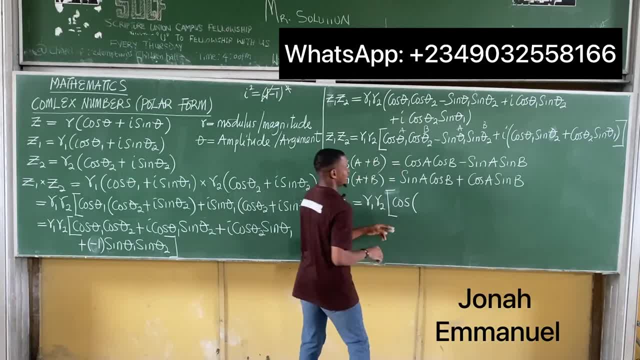 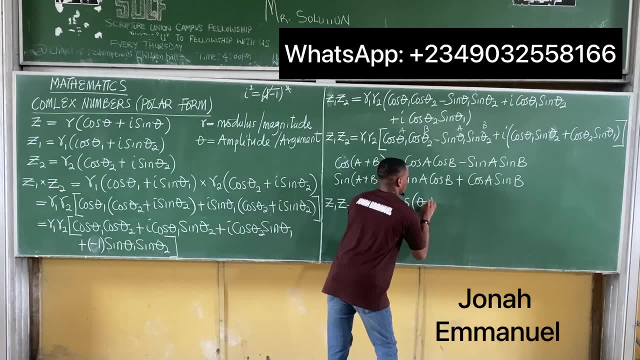 That means I can write this as being cos into. in this case it was a and b, but in this case I used theta 1 and theta 2, so it becomes cos: theta 1 plus theta 2.. Theta 2, the same concept. all right, so that's just this. 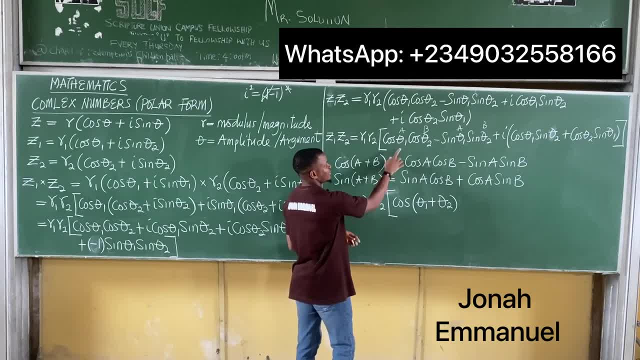 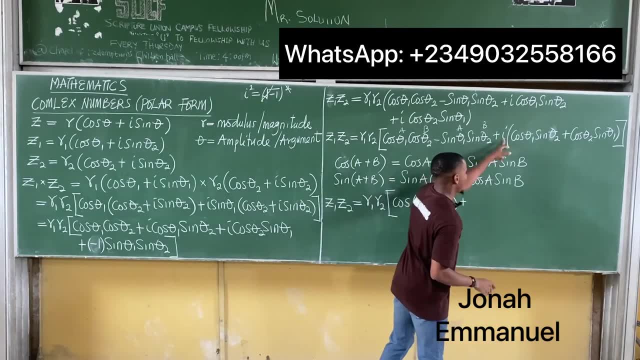 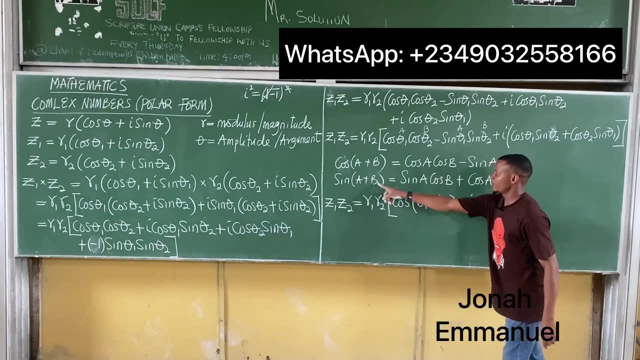 That's just writing this one here in this form, but in this case I'm using theta 1 and theta 2, and not just a and b. So plus my next time says i, so I have i Similarly for this one here. if you observe this, I have that sin. a plus b is equal to. 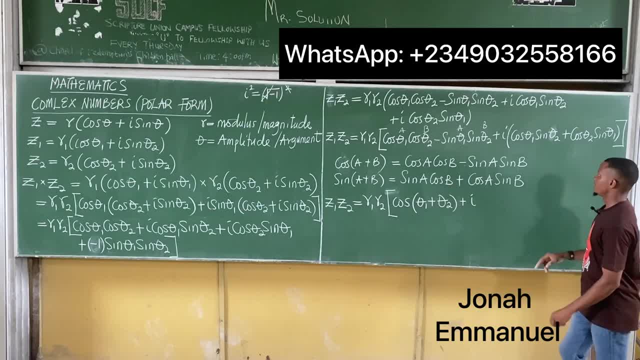 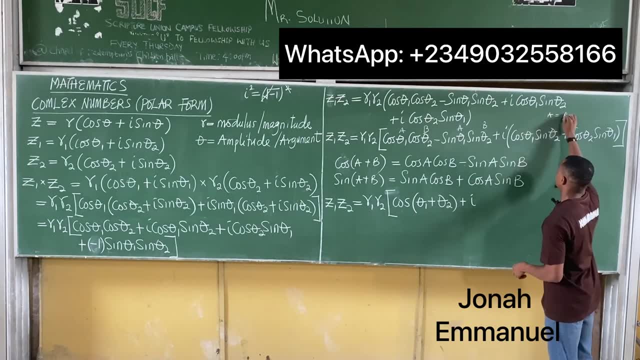 sin a cos b plus cos a sin b. That's the same thing as this one. here. As you can see this, let's call a to be equal to theta 1, and b to be equal to theta 2.. So that would be sin theta 1,, which is this, cos theta 2,, which is this: 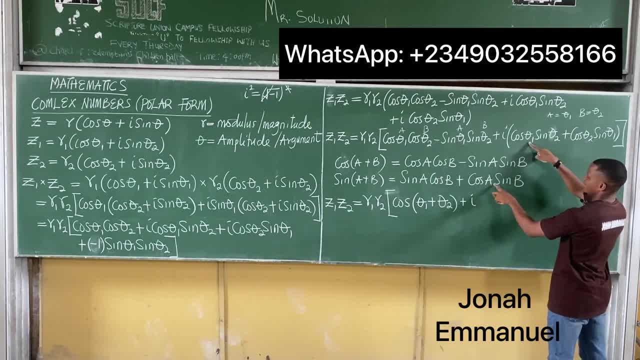 plus cos theta 1,, which is this, sin theta 2,, which is this: All right, so this is. these two are the same thing, Although they're not arranged in the same form, but it's the same thing because this is called the commutative law of mathematics. 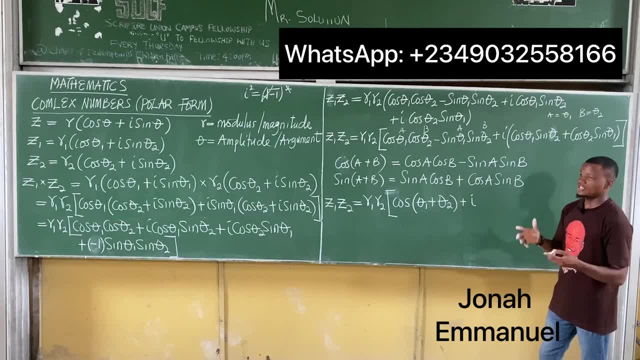 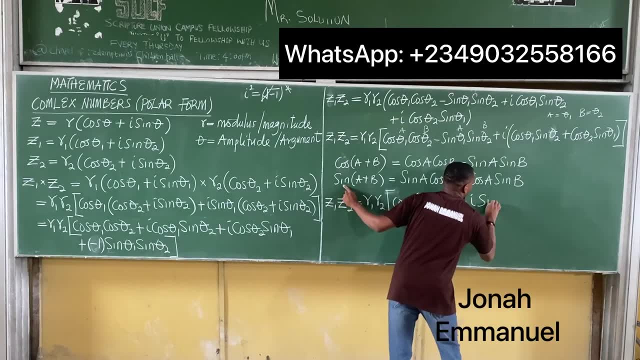 So, although they're not arranged perfectly as this, they're doing the same thing. This is their multiplying. So hence this one here, this whole thing here can be rewritten as sin. Now we said: theta 1 is a, so it becomes sin, theta 1 plus b, theta 2.. 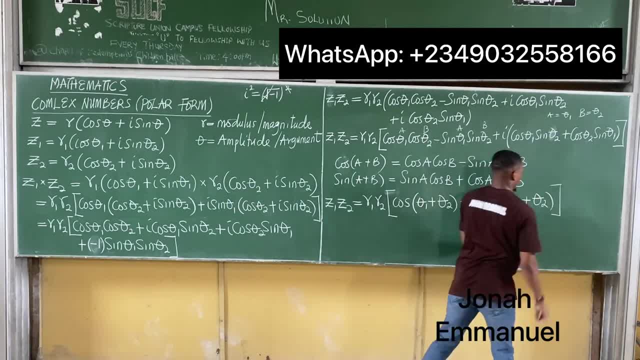 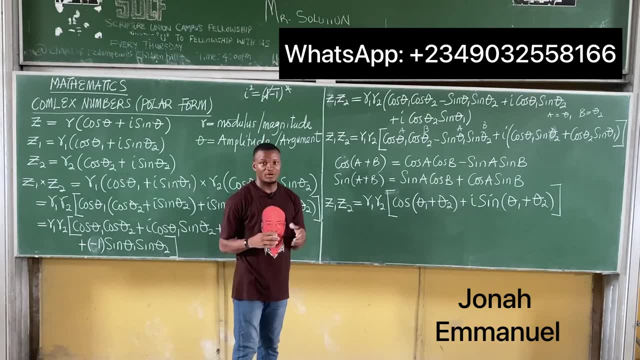 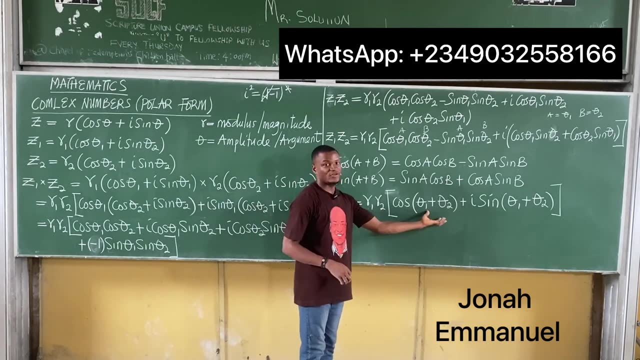 So theta 2, I have this All right, so this becomes the answer. So that means, if I'm multiplying any two complex numbers in polar form, the idea is simple: Multiply, Add their modulus, open bracket, cos, add their argument or their amplitude. 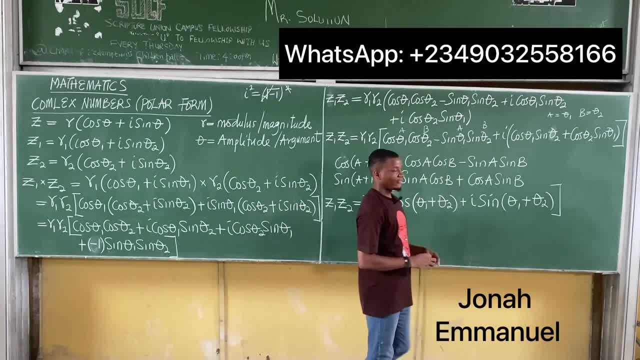 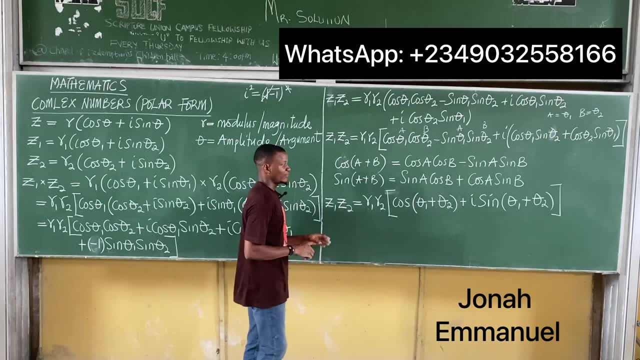 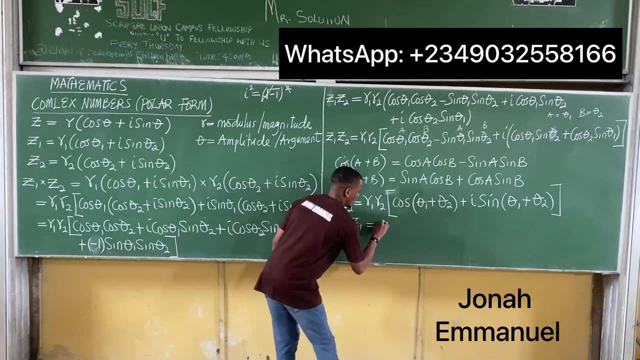 plus i sine, add the second value of the amplitude and etc. So this is simply how we multiply two complex numbers. We'll take a quick example and we'll do this. So with this now example. So example, let me say I had z1 as being equal to 3 into cos 45,. 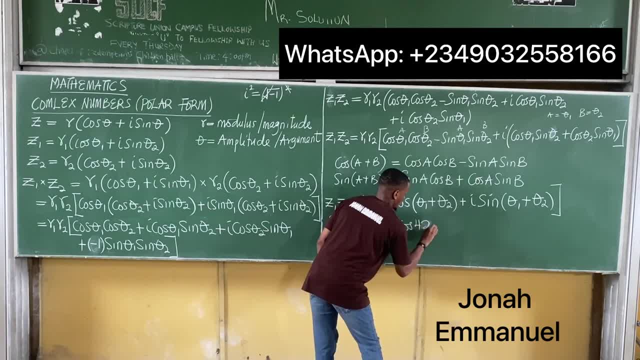 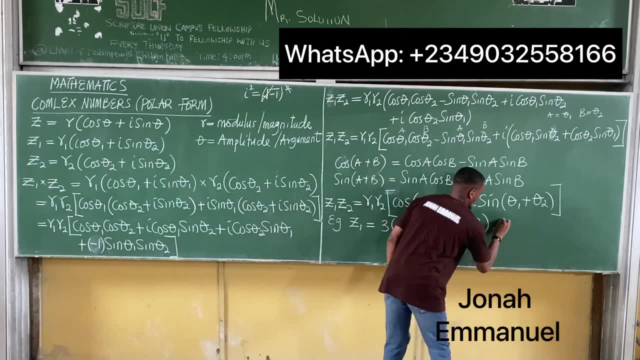 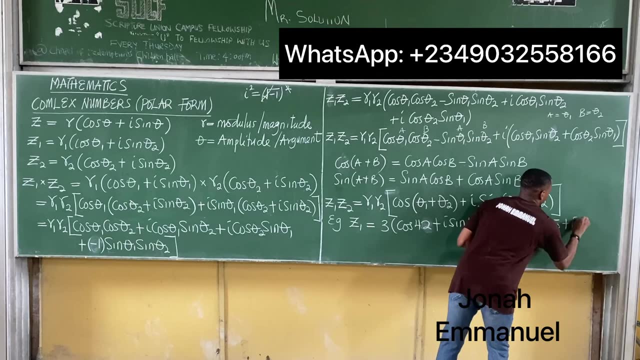 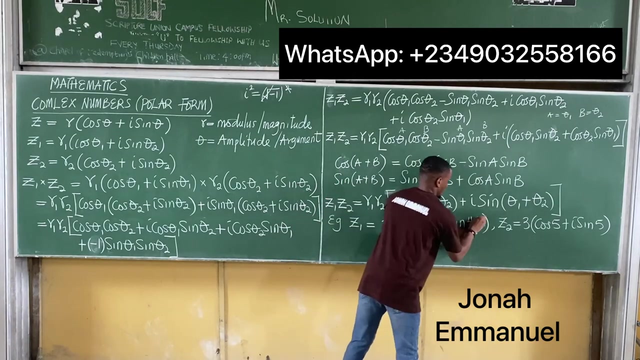 or let's say 42, plus i sine 42. And I had z2, z2 as equal to 3 into cos 5 plus i sine 5.. And I'm actually fine. of course this is in degrees. So in degrees, in degrees, in degrees and also in degrees. 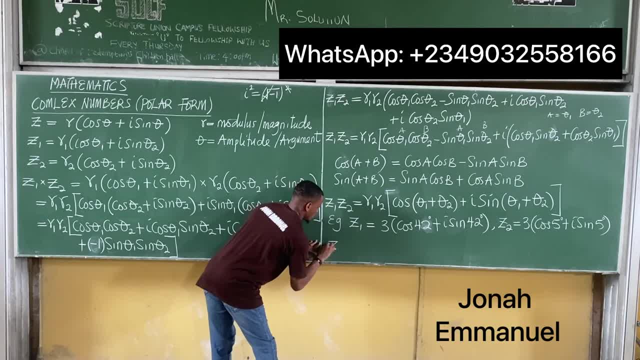 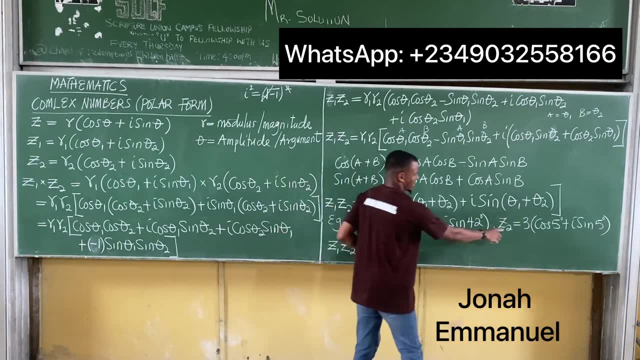 So I have this, So I have this, So I'm asked to find the value of z1 and z2.. So z1, z2 will simply be equal to r1, r2.. r1 here is 3.. r2 here is 3.. 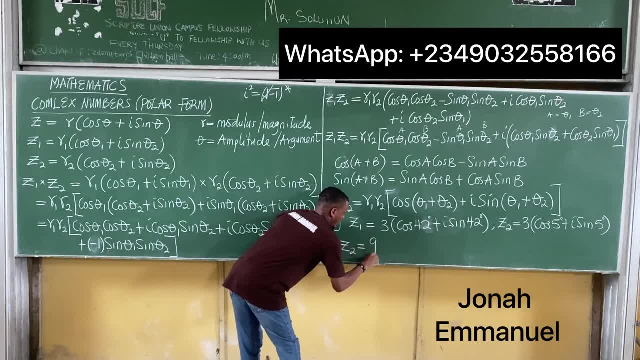 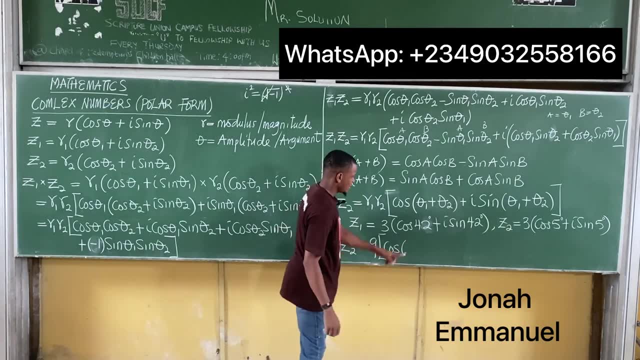 Okay, That becomes 3 times 3, which is what there 9 into. I will now have cos of. in this case, theta 1 is 42. Theta 2 is 5.. So it becomes 42 plus 5.. 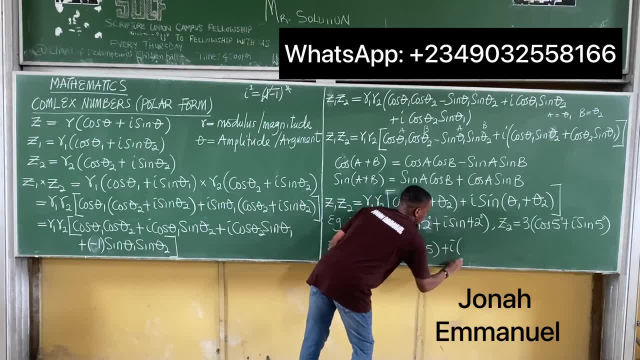 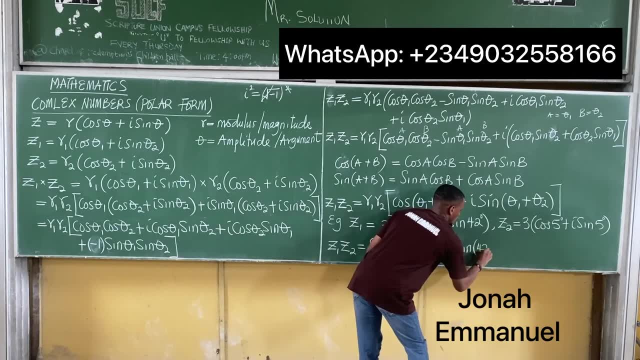 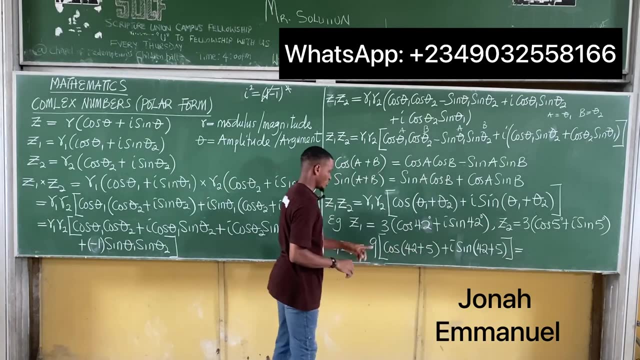 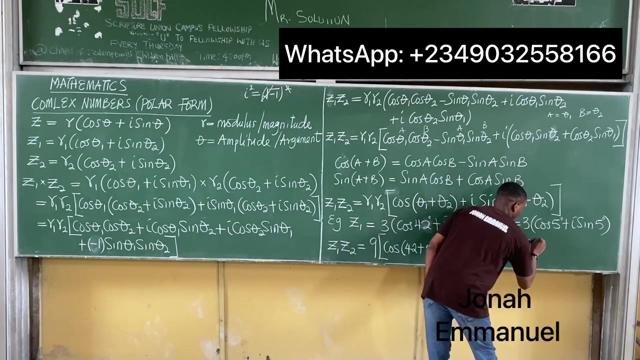 42. Plus 5 plus i. into sine, of course, theta 1 here is still 42. So 42 plus theta 2 here is still 5.. So I have 5, all in degrees And my final is going to be equal to 3 times 3,. 3 times 3 here, which is 9, into I have cos 42 plus 5,. 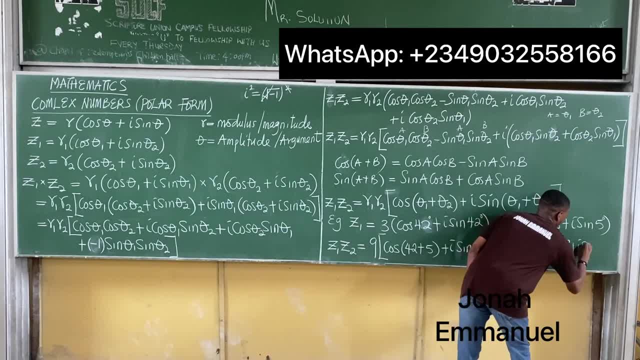 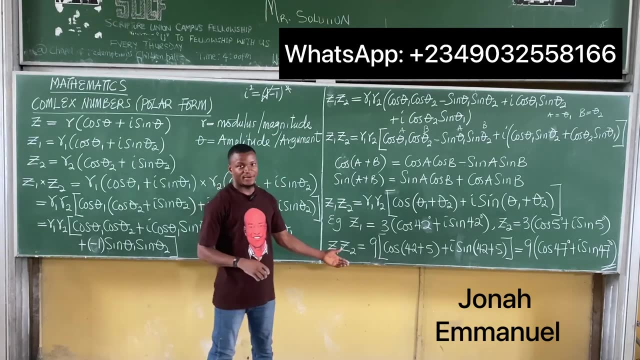 47 degrees, plus i sine for 2 plus 5, 47 degrees. So this would be my final answer after multiplying these two complex numbers in polar form. So this is how we multiply complex numbers in polar form, All right. 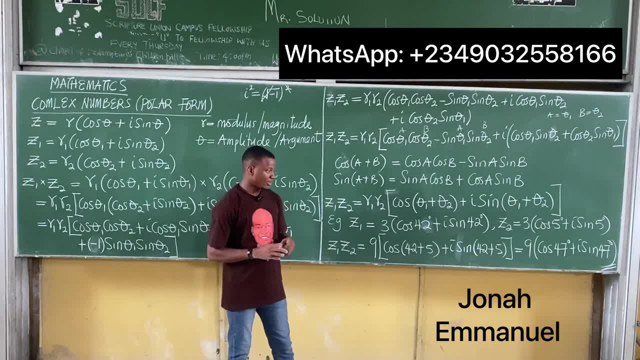 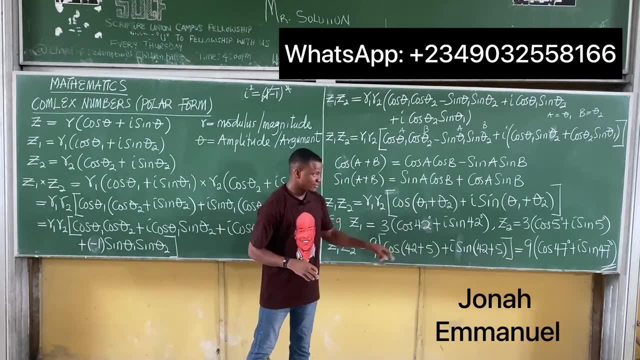 All right, so this is how we multiply complex numbers in polar form. So let's look at Um The multiplication of complex numbers in polar form. But this one here was in degrees, So let's What about What if it is in radians? 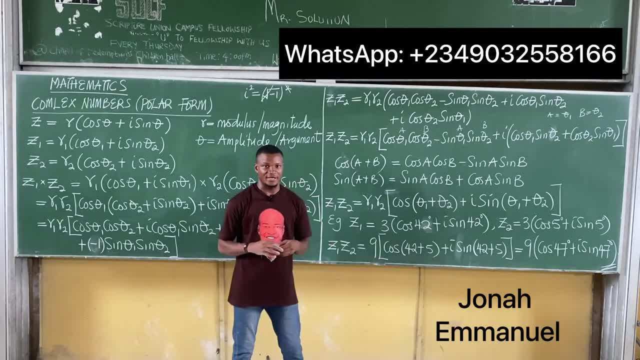 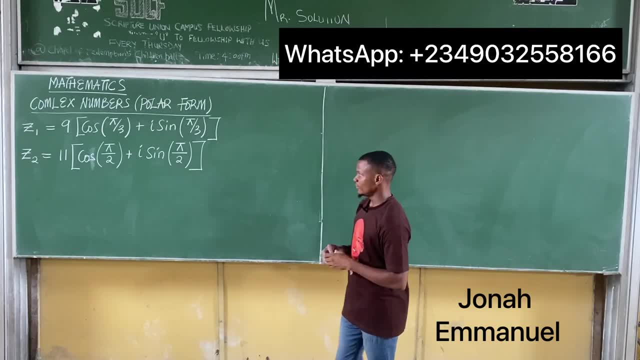 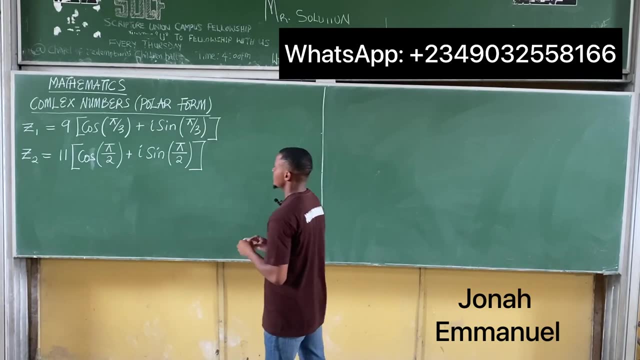 Look at how to also multiply complex numbers when they are in radians in our next example. All right, let's take a second example. So let's say we are given z1 as being equal to 9, cos theta over 3 plus i sine. 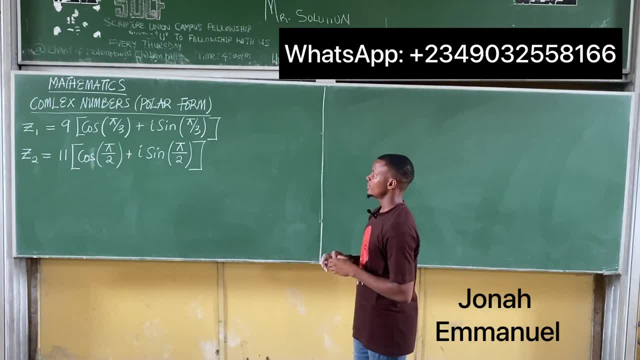 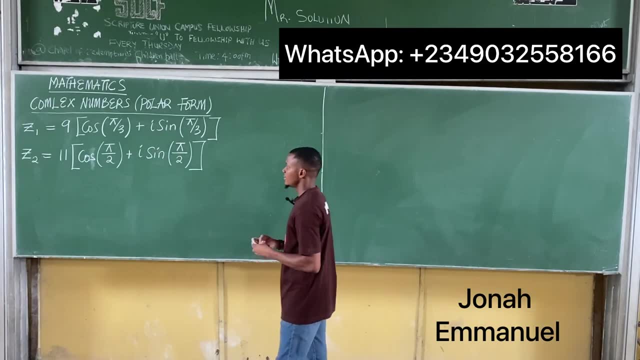 So let's say we are given z1 as being equal to 9. into cos pi over 3 plus i sine pi over 3.. Um, And z2 as 11 cos pi over 2 plus i sine pi over 2.. 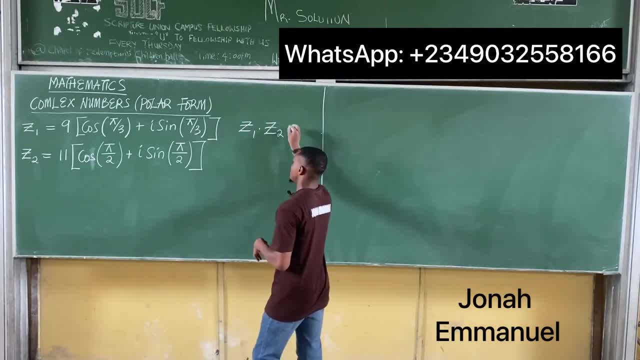 And we're asked to find the value of z1 multiplied z2.. So how do we solve this? Uh, remember that we said: Let's recall something, Recall that we said um z1 z2.. We said: z1 z2 is equal to r1, r2 into cos. 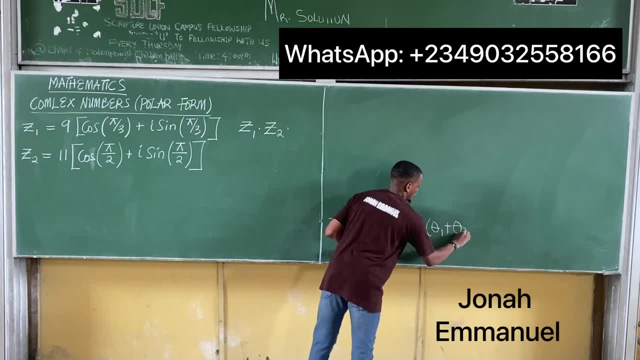 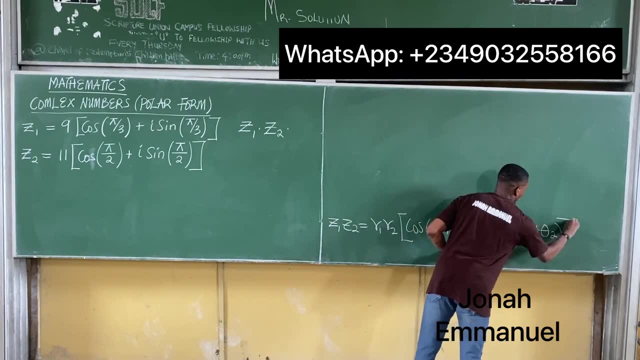 cos of theta 1 plus theta 2, um plus i sine theta 1 plus theta 2.. We had this one here, So the idea was simple That z1 z2.. z1- z2 is equal to multiply the. 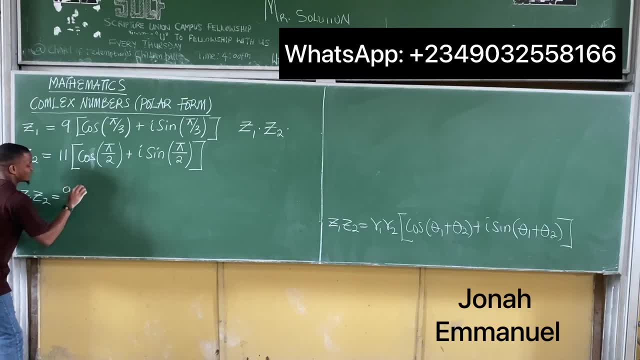 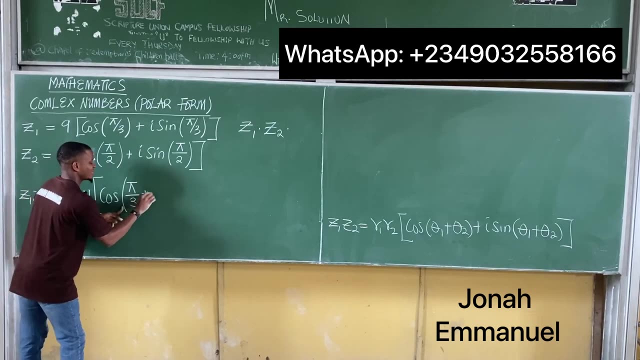 the two uh modules, So 9 times 11, into um cos of theta 1. plus theta 2. That becomes the angles. So the angle now is in terms of radians, no longer degrees, But I'm still adding them anyways. 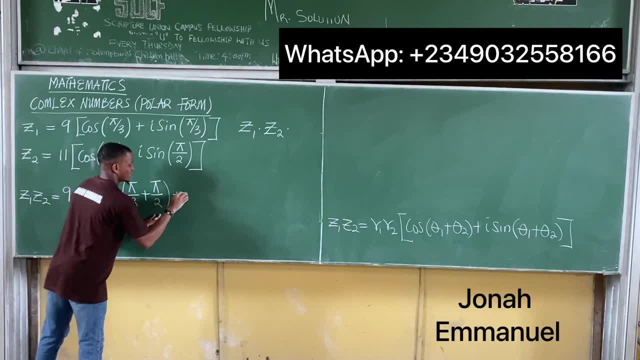 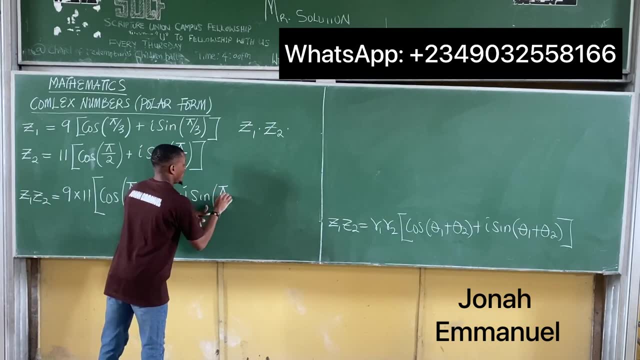 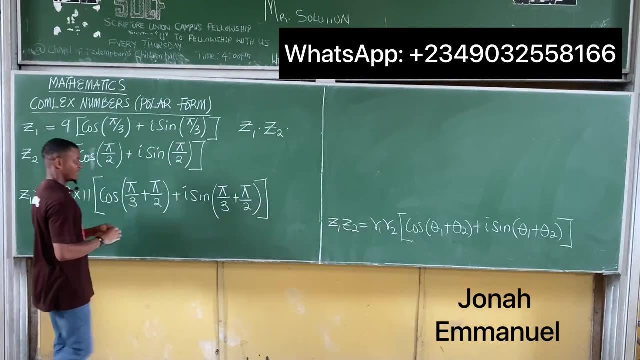 So this all over 2.. So add this Plus i sine Um, having this one here, Theta over 3. Or pi over 3 plus pi over 2.. So it's quite simple, Just add these And let's see what we get. 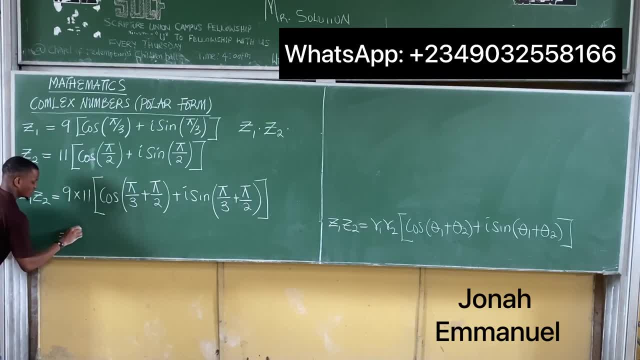 So if we work on this now, this is equal. Also, 9 times 11 is 99.. 99 into I'm having cos. Take the LCM here. My LCM here, 3 and 2, is 6.. 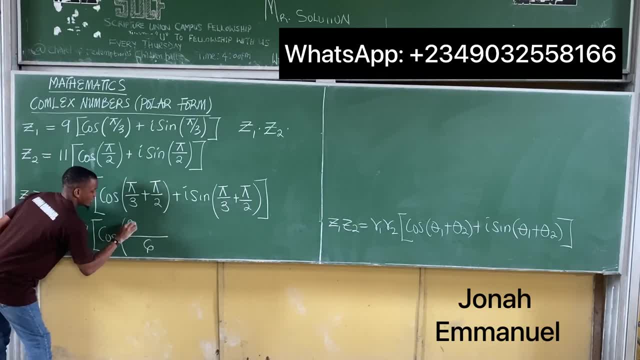 So 6 over 3 is 2 times pi is 2 pi. plus 6 over 2 is 3 times pi, is 3 pi. So I have this Plus i sine. Take the LCM of 3 and 2.. 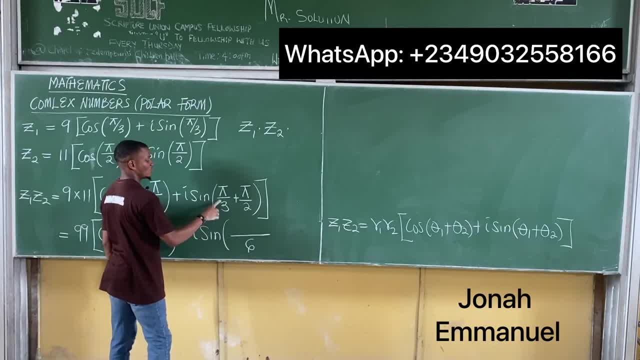 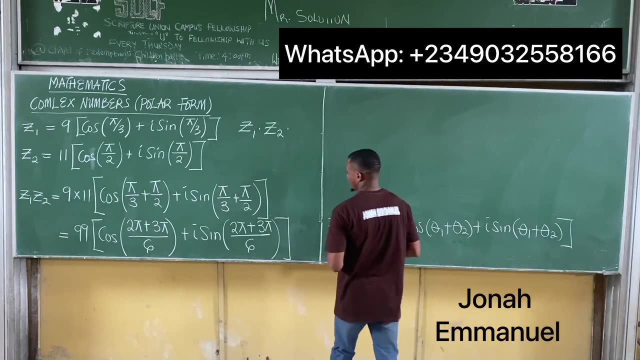 And that again is 6.. 6 divided by 3 is 2 times pi is 2 pi. plus 6 divided by 2 is 3 times pi is 3 pi. So we have this Alright. So it means that z1, z2 is simply equal to 99 into cos. 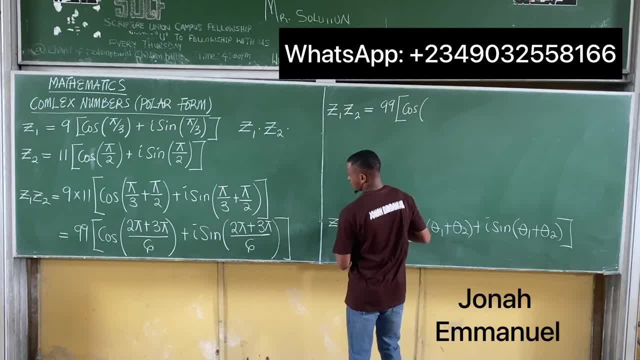 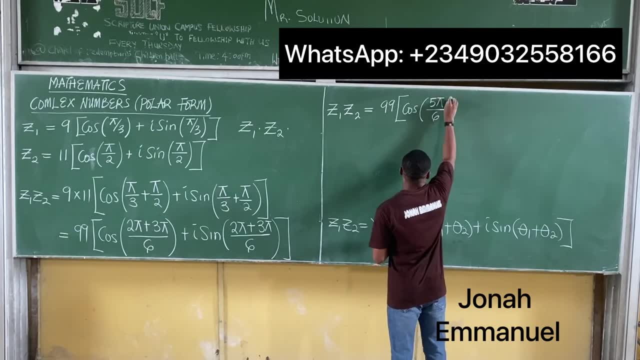 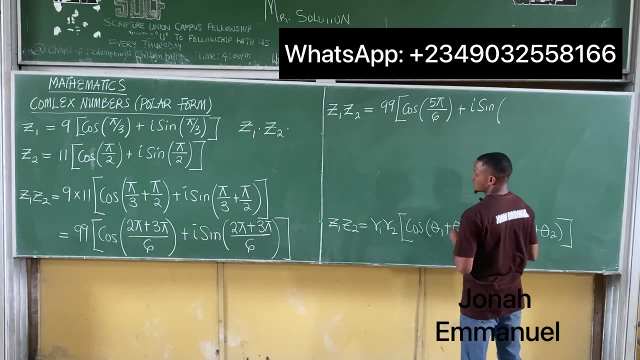 Um, Into cos. 2 pi plus 3 pi gives you 5 pi all over 6.. So I have this Plus i sine. I have 2 pi plus 3 pi. That's about 5 pi all over 6.. 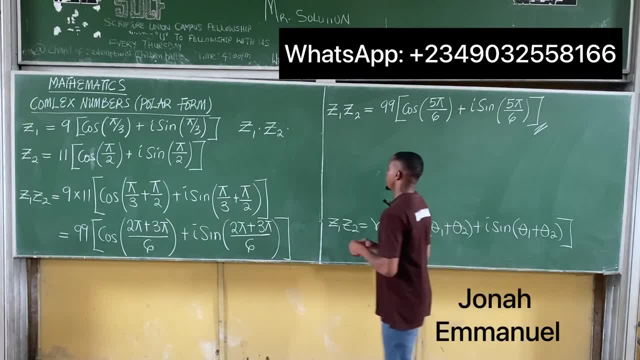 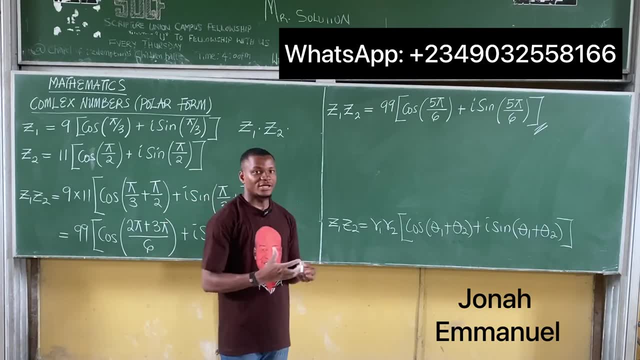 So I have this, So this becomes the answer in radians. So this is the value of z1, z2.. In radians, If you ask to provide this value in terms of degrees, Alright, You say, leave your answer in terms of degrees. 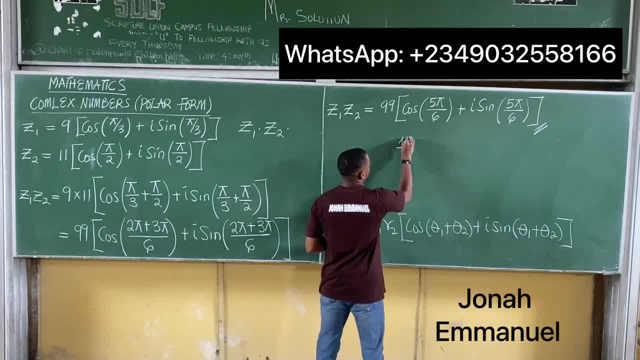 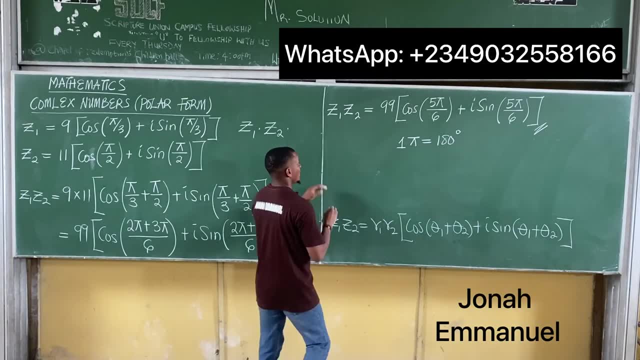 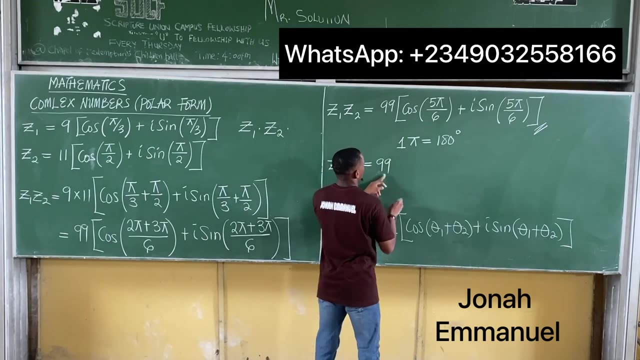 What do you do? Very simple. We said: 1 pi is equal to 180 degrees, So simply replace pi as 180 degrees. there We'll have that z1, z2 is equal to 99 into cos, Um, Into cos. 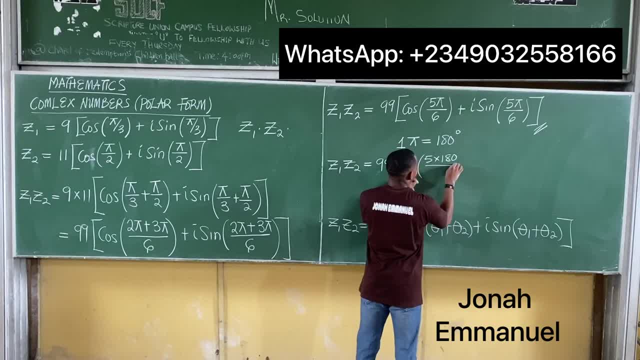 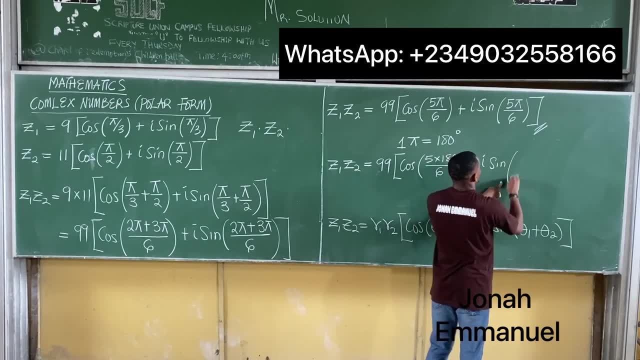 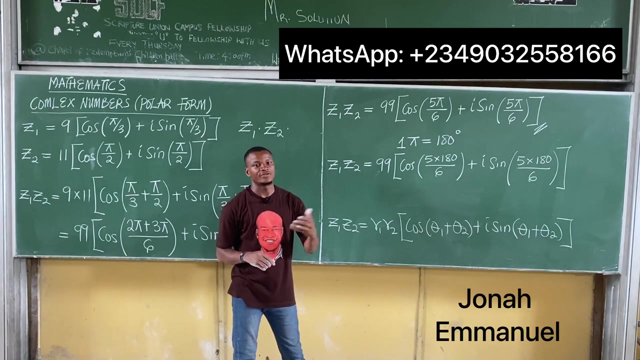 5 times 180.. That's pi 180 all over 6.. Plus i sine 5 times pi, 5 times 180 over 6.. So we have this value. Now let me clarify something for you. The value of pi in angular measurement is 180 degrees. 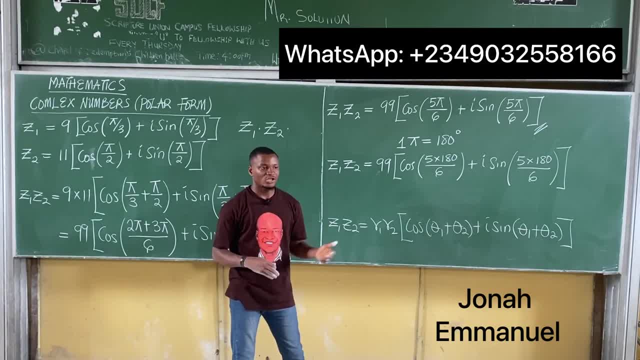 But in other branches of mathematics, like We'll talk about mesuration, Pi is equal to 22 over 7.. That's like 3.14, whatever there. Alright, But that's not in this case In terms of angular measurement, degrees and radians. 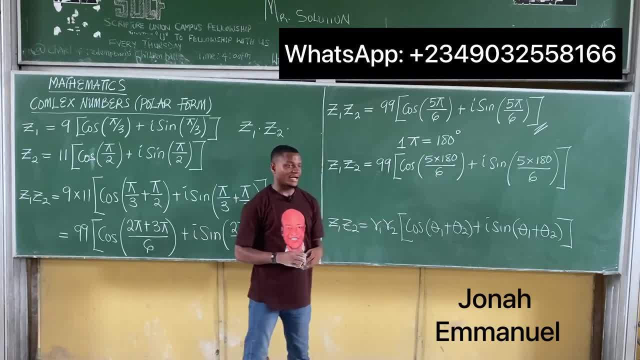 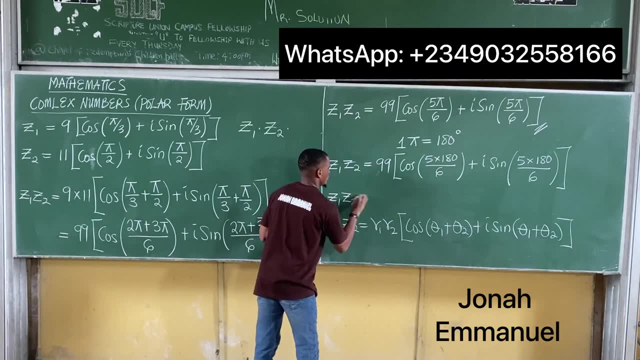 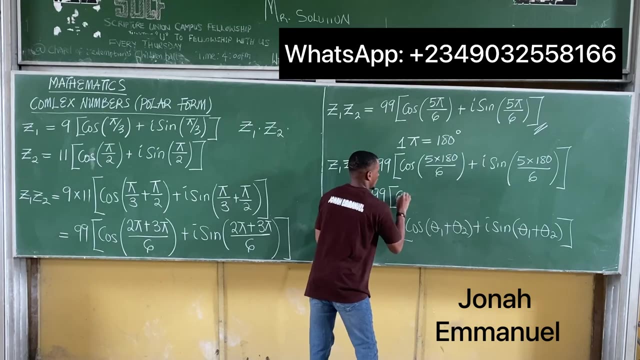 Pi is equal to 180 degrees. We talked about this in a previous class. Alright, Let's simplify this. So it means that my final answer, z1, z2, will be equal to 99, into I'm having this as cos: 6 here 1,, 6 here 30. 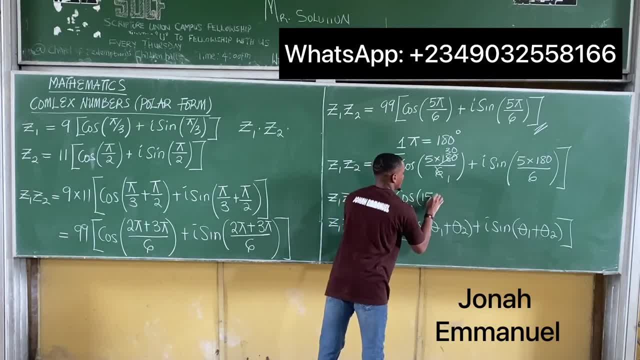 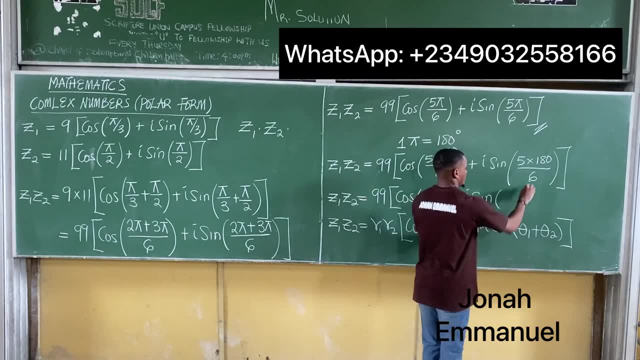 5 times 30 is 150.. So 150 degrees. This plus i sine 6 here 1,, 6 here 30.. 5 times 30 is 150 degrees. Alright, So this becomes the value of z1, z2.. 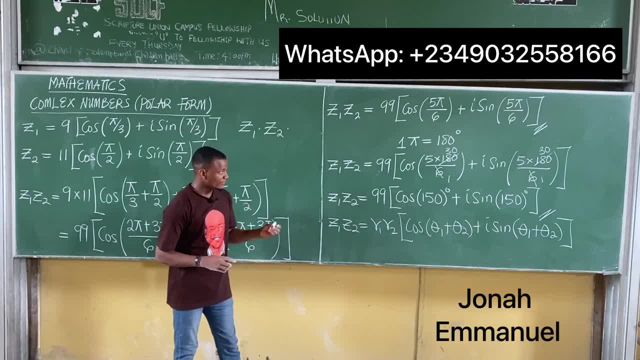 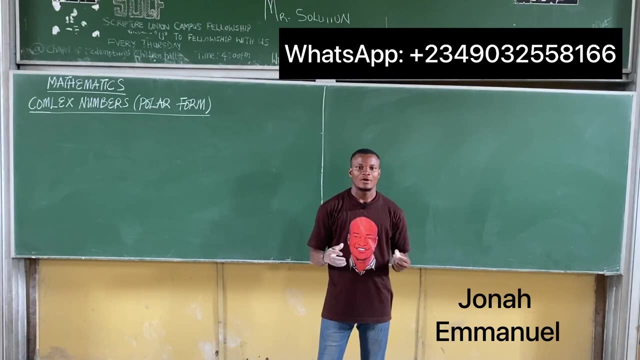 In terms of degrees. Alright, So this is how we solve the multiplication of complex numbers in polar form. Next up, let's look at the division of complex numbers in polar form. Alright, So let's now look at how to divide complex numbers in polar form. 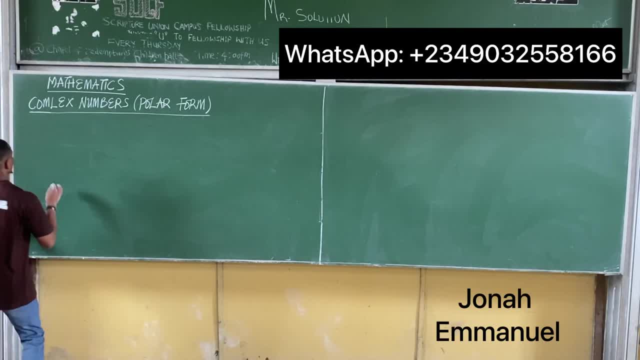 So let's look at the division of complex numbers in polar form. Let's say we are given our first complex number in polar As z1 equal to r1 cos theta1 plus i sine theta1.. And z2 being equal to r2 cos theta2 plus i sine theta2.. 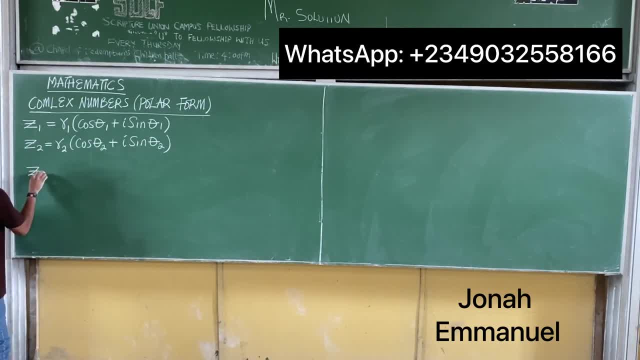 And we have to evaluate the equations z1 over z2.. So for this one here I won't really go into the derivation of the formula, as I did for multiplication. So I'll just give you the final answer of how it works And we can take some few examples and proceed. 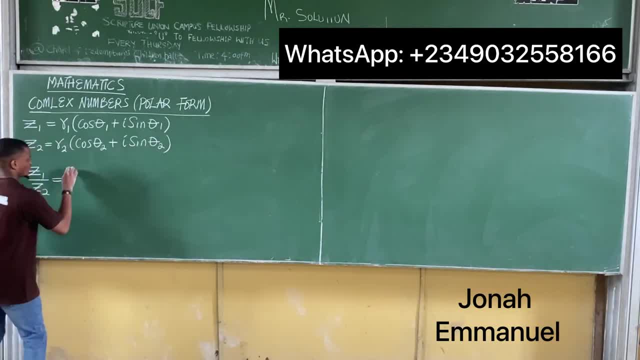 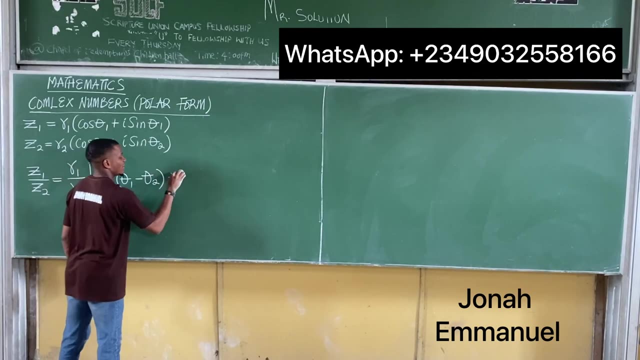 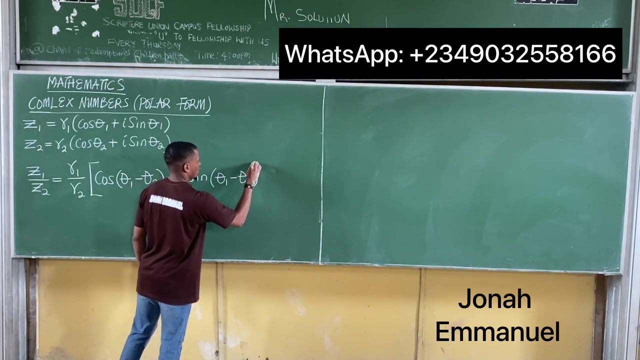 z1 over z2. in polar form is equal to r1 over r2 into That becomes cos of theta1 minus theta2 plus i. Okay, So we have sin theta1 minus theta2.. So we have this case here. We have this case. 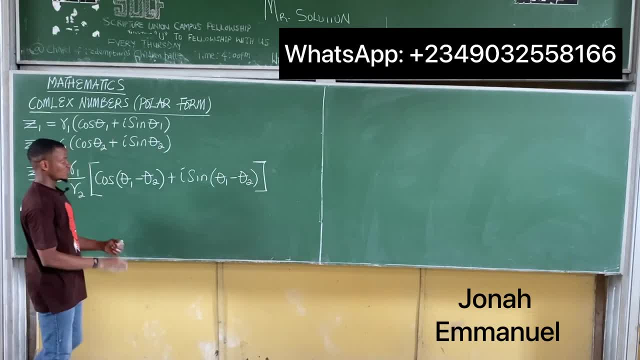 Alright. So this is how. This is the formula that helps us to do the division of complex numbers. Alright, It's kind of similar to multiplication, Just that for multiplication these two, I'm actually multiplying them, But for division, I'm dividing them. 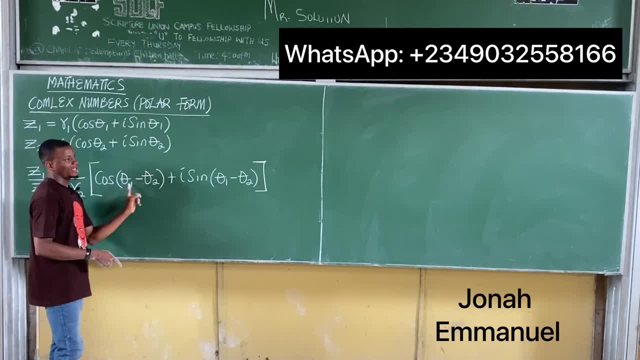 These two for multiplication. I am adding the angles, All the amplitude, all the arguments for multiplication. I am subtracting the angles and not adding them. Alright, So that's how this works. Let's get an example. Let's say example 1.. 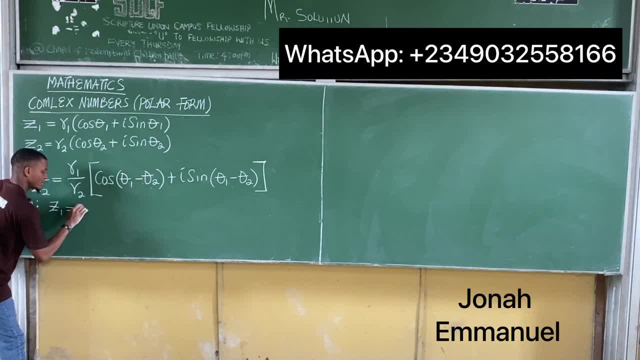 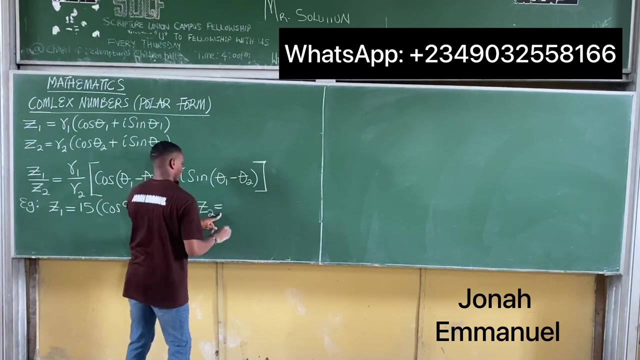 z1 is equal to 5.. Or let me do something like 15.. 15 into cos 9 degrees Plus I sine 9 degrees. And then I have z2 has been into 3.. Has been equal to 3 of cos 5 degrees plus i sine 5 degrees. 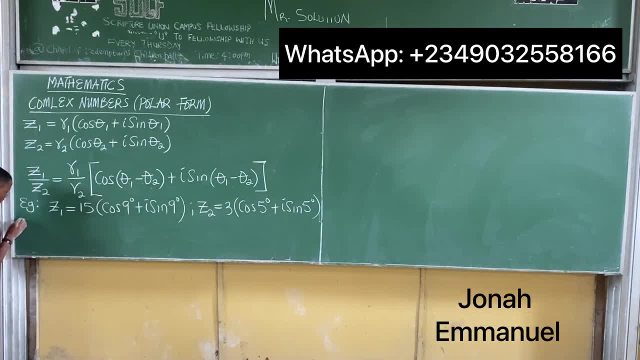 So I have this. I'm actually finding z1 over z2.. Obviously, z1 over z2 will be equal to, We said, divide the Modulus That becomes 15 over 3 into cos, Subtract the angles 9 minus 5.. 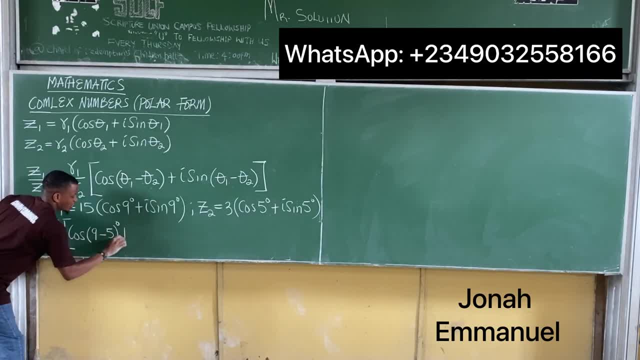 So I have 9 minus 5 all in degrees, Plus i sine 9 minus 5.. So I have 9 minus 5 all in degrees. If I work on this, 15 divided by 3 gives you 5.. So I have 5.. 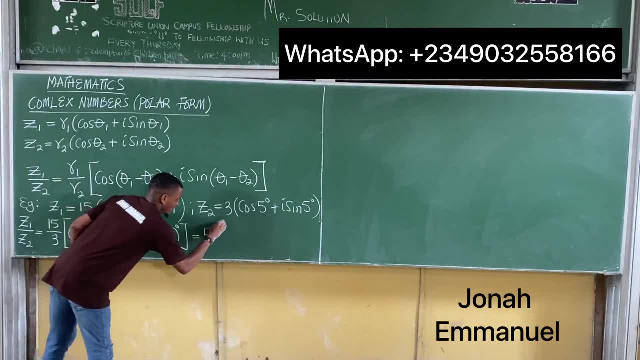 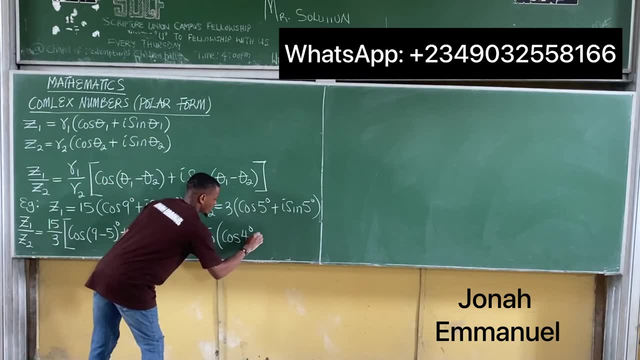 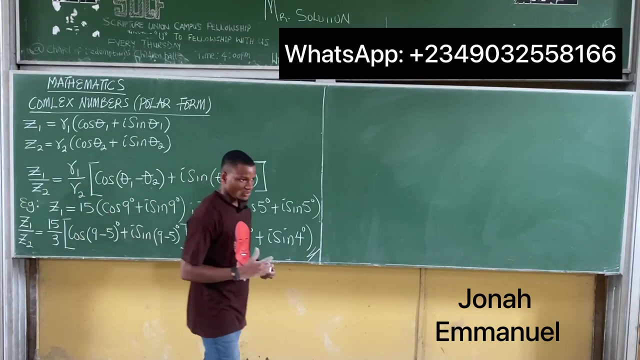 Into this one here. That becomes cos: 9 minus 5 is 4 degrees Plus i sine 9 minus 5.. Still another 4 degrees, Alright. So this is how we divide complex numbers in polar form We look at: 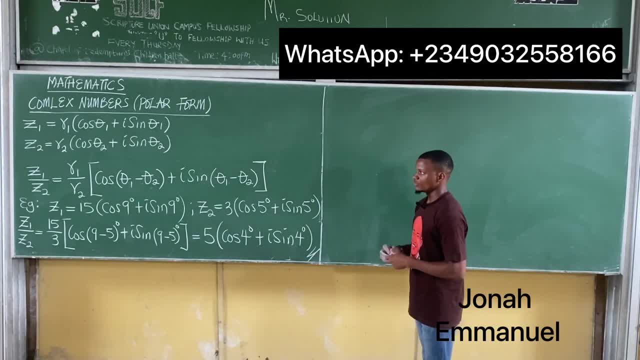 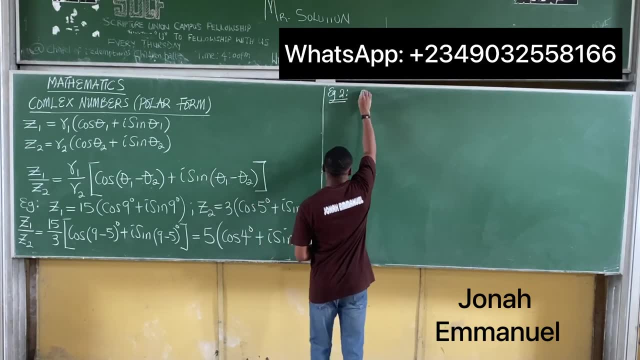 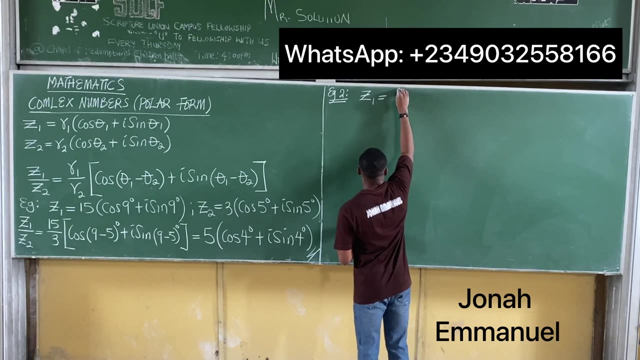 Now, this was working with degrees. Let's work with gradients And then we'll. We'll be done with this. So example 2.. So example 2.. Let's say z1 is equal to 11.. 11 into cos, pi, all over 2.. 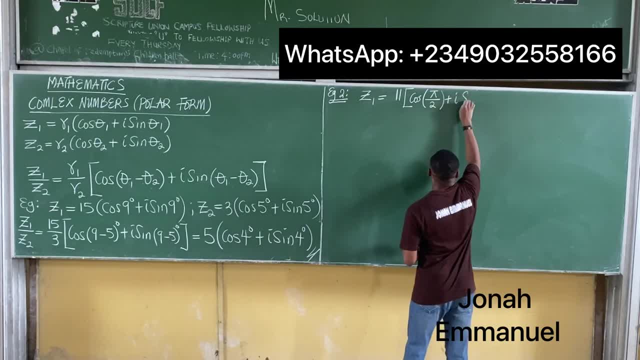 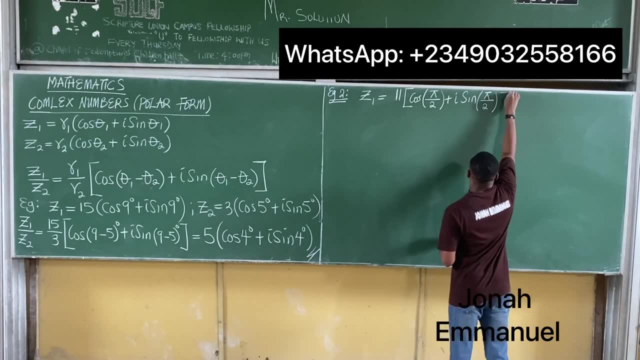 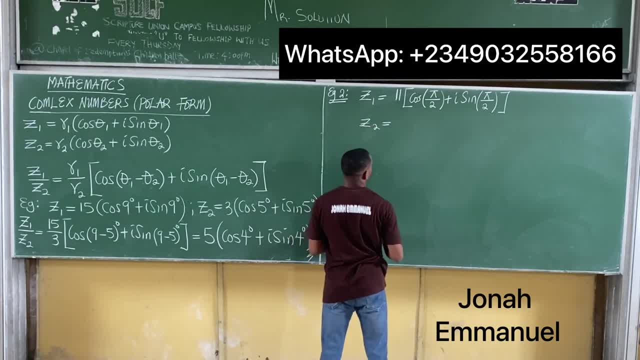 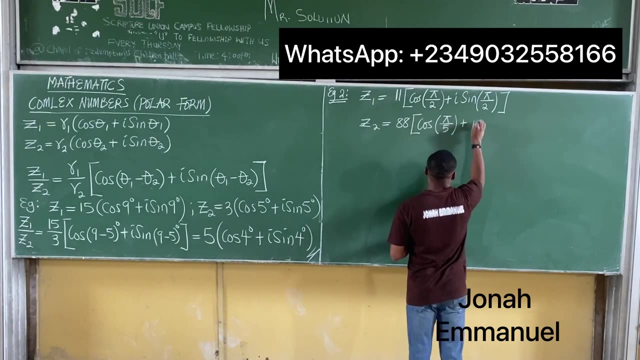 So we have z2 as being equal to 88.. 88 into cos pi all over 5.. Plus i sine pi over 5, let's say we had this one. here we actually find the value of z1 over z2, so from here, 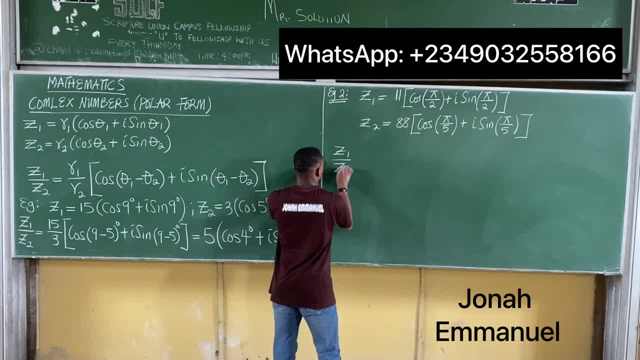 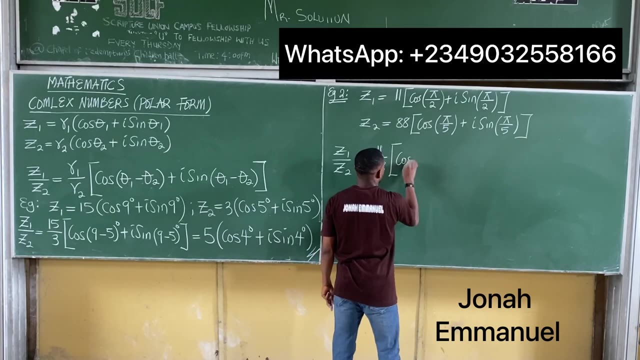 z1 over z2 will be equal to we said: divide this so it becomes 11 all over 88, so z1 over z2, that's r1 over r2 into cos: theta1 pi over 2 minus theta2 pi over 5 plus. 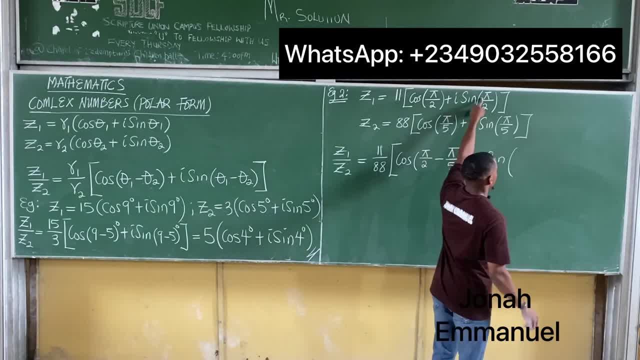 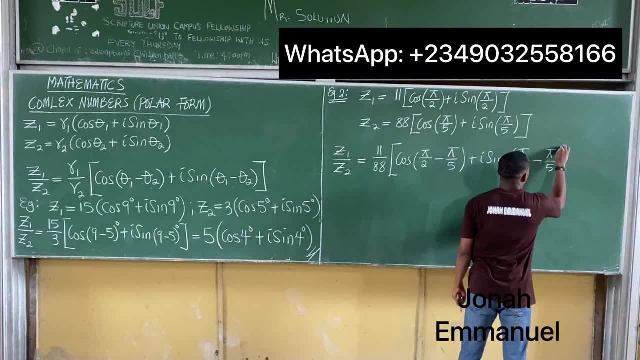 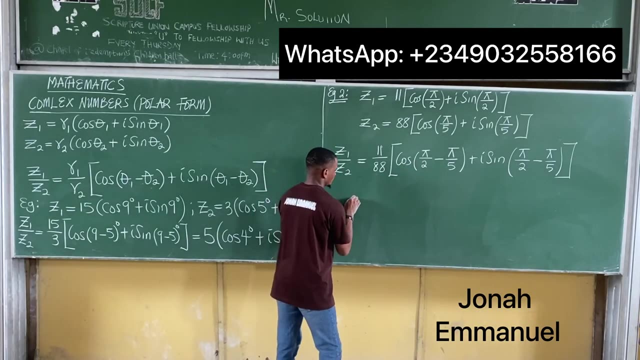 i sine theta1 pi over 2 minus theta2 pi over 5, so I have this expression now. I don't have to work on this. this will be equal to. that's equal to to lower stem: 11 here is 1,. 11 here is 8, that gives you. 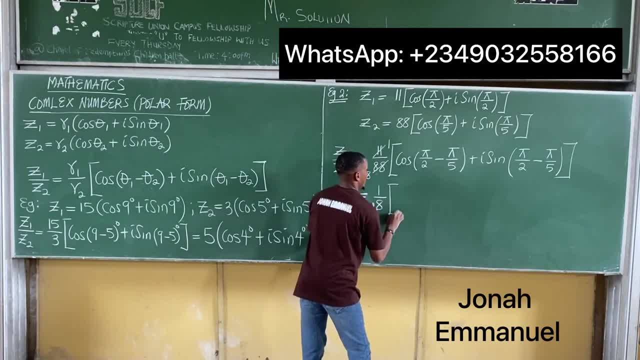 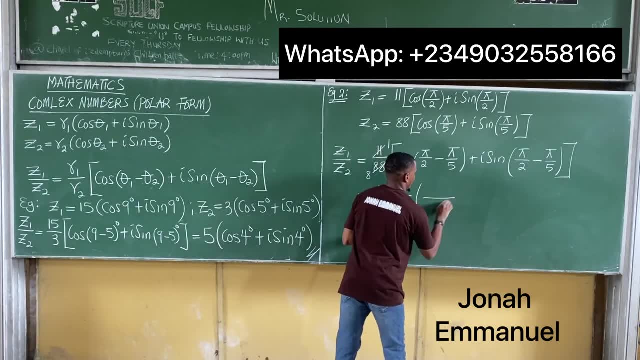 1 over 8 into. I have this as cos. take my LCM here. the LCM of 2 and 5 is 10, my LCM is 10. sorry, my LCM here is 10. so 10 divided by 2 is 5 times pi. 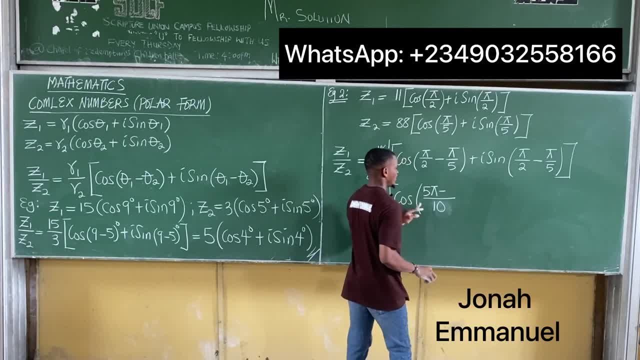 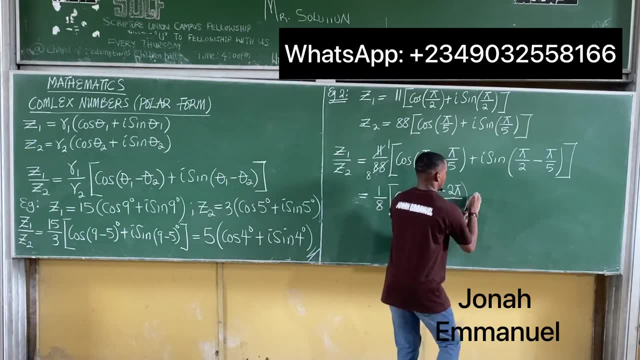 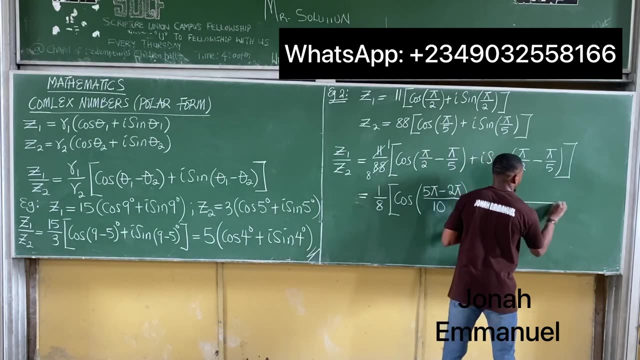 is 5 pi minus 10 divided by 5 is 2 times pi is 2 pi. we have this one here plus i sine. we have this one here: LCM of 2 and 5 is 10, so 10 divided by 2 is 5 times pi. 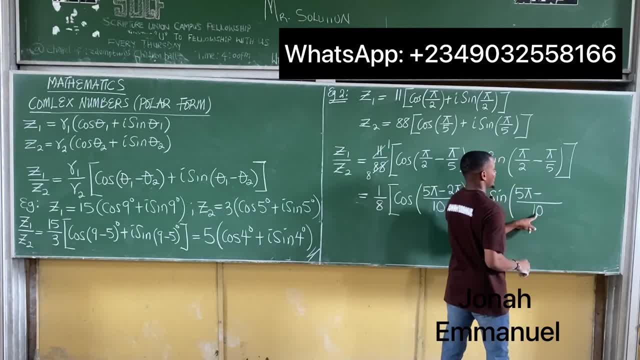 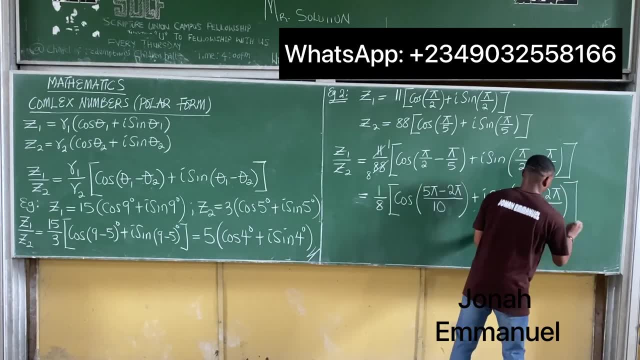 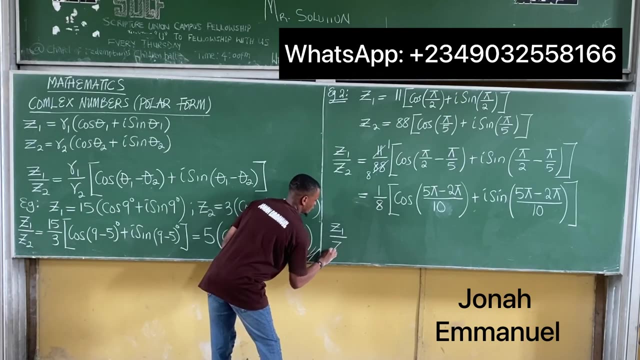 is 5 pi minus 10. divided by 5 is 2 times pi is 2 pi. so we have this one here, alright. so that means that z1 over z2, z1 over z2. on final simplification this gives you: 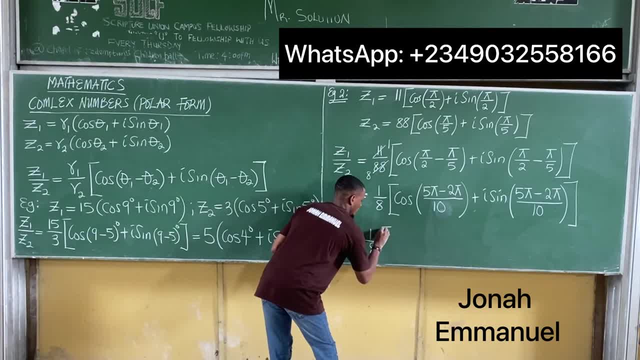 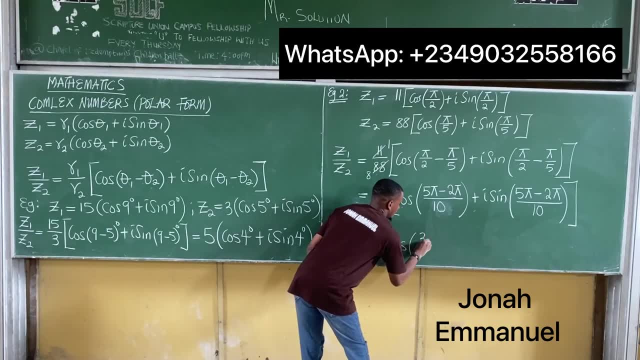 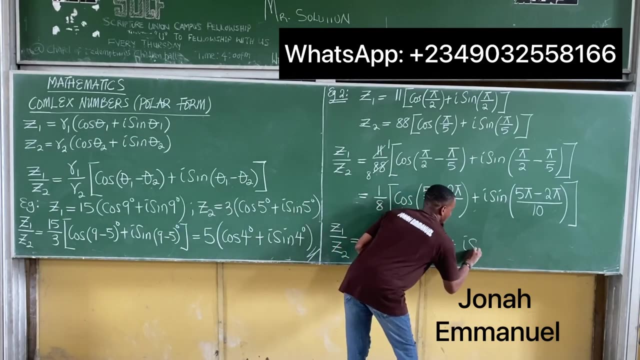 1 over 8 into. I'm having this as cos, so cos work on this. 5 pi minus 2 pi gives you 3 pi all over 10, so I have this plus i sine. 5 pi minus 2 pi is 3 pi all over 10. 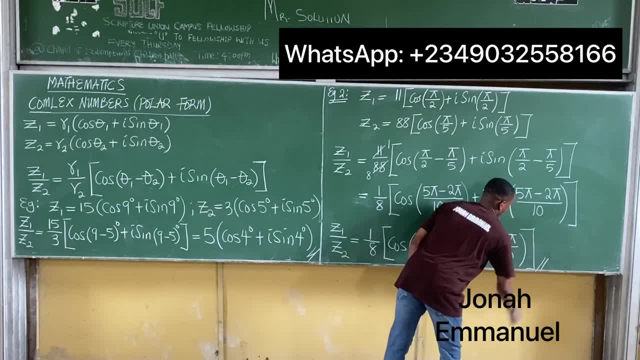 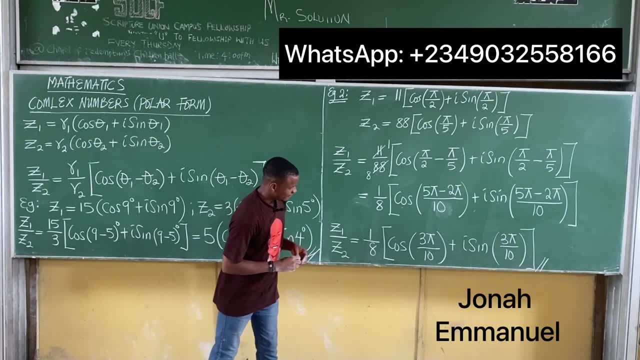 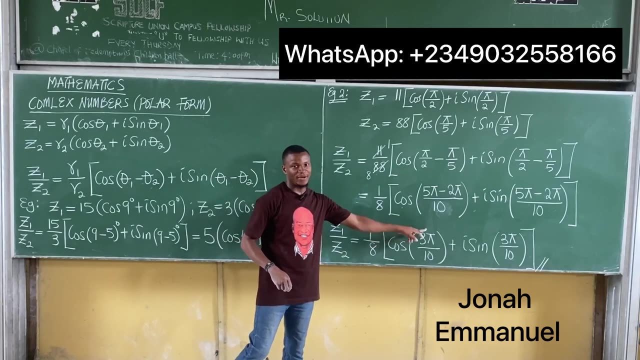 so I have this answer, alright. so this is how you divide two complex numbers in polar form, alright, if you want to? now, of course, this one here is done in radians. that's why we use pi. if you want to convert this answer to degrees, simply substitute pi as 180. 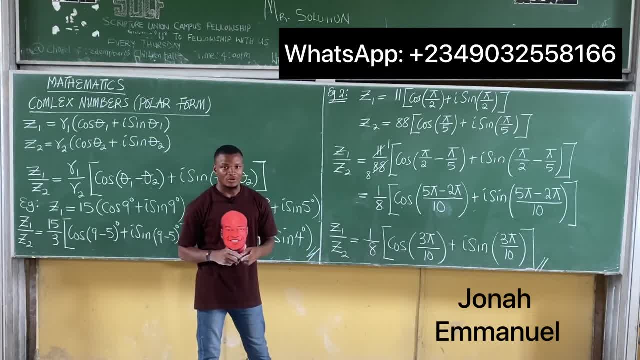 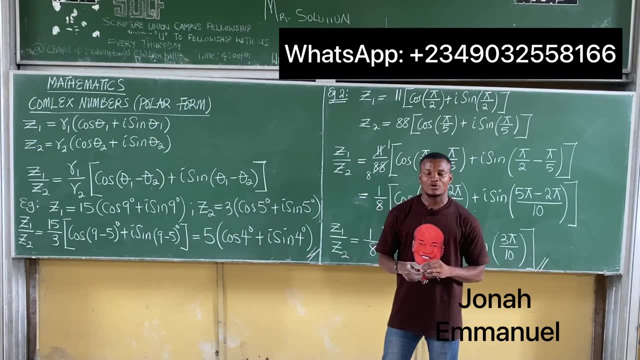 and do your thing, alright. so this is how you do it: solving- alright, and then you have your answer, alright. so this is how we do this work. before we go, one final thing I'll show you is how to convert a complex number. 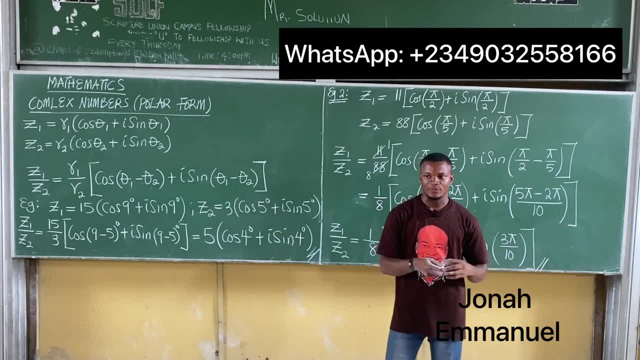 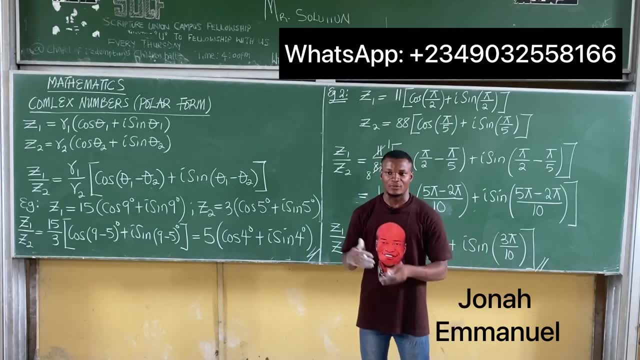 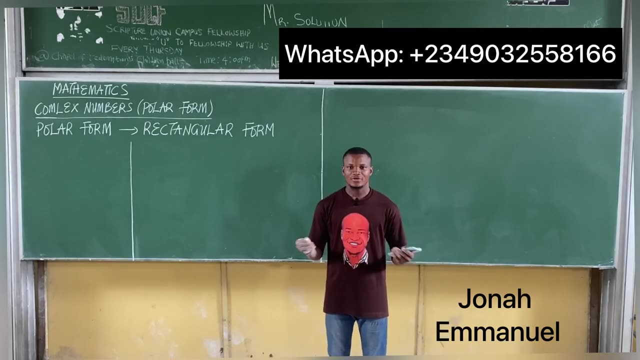 from polar form to rectangular form. alright, we've seen how to convert from rectangular form to polar form. now let's look at how to convert complex numbers from polar form back to rectangular form, and then we'll call it a class, okay? so finally, let's look at how to do this. 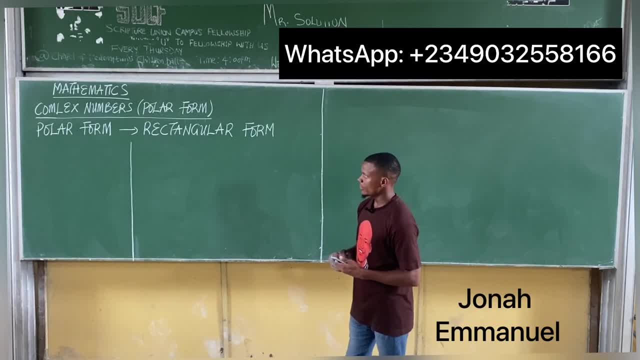 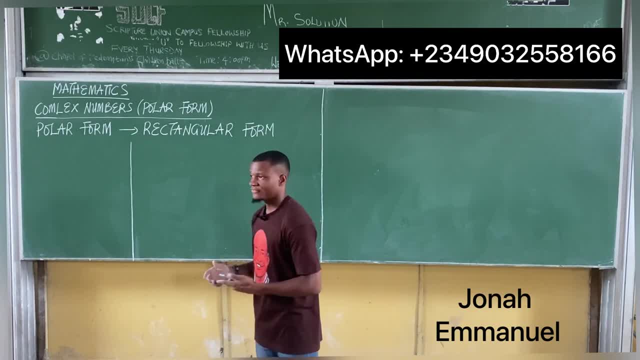 rectangular form- or you can see the cartesian form- to the secular or polar form. but for this video we looked at how to convert it from polar form back to the rectangular or cartesian form. but before we do that, let's take a very simple example, a brief one. 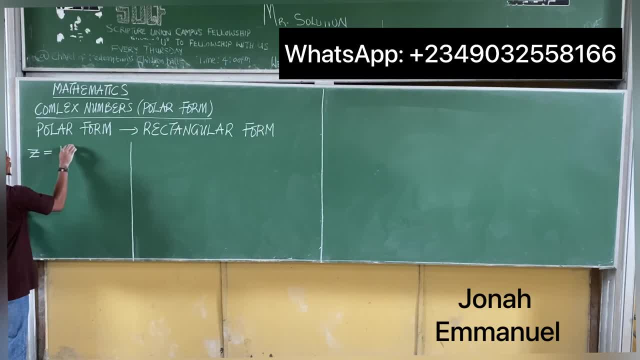 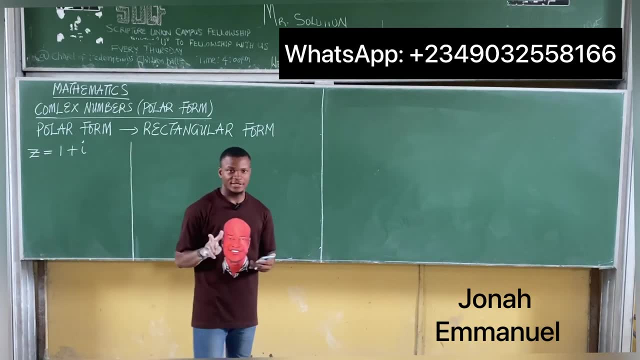 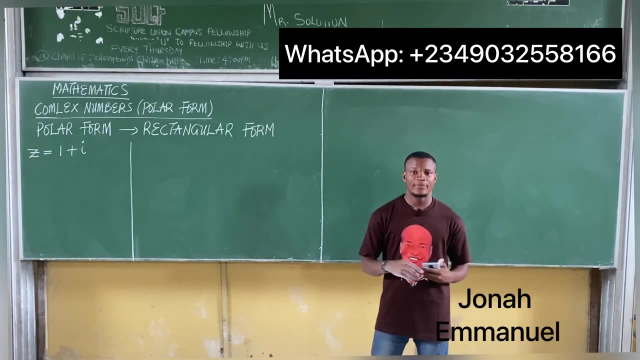 triangular form if a complex number z is equal to 1 plus i, for instance. now to convert this one here to a polar form, we need to find two things. The first one, we said, is the magnitude or the modulus of this complex number. The second one we said is the. 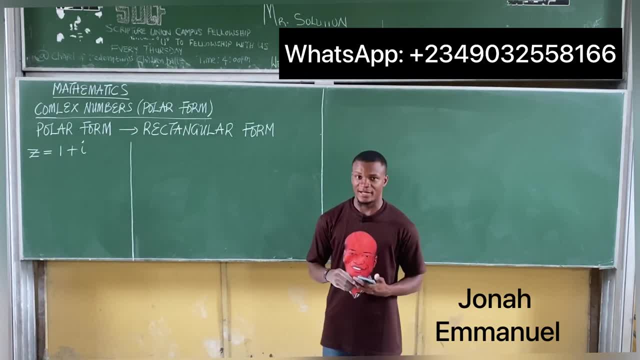 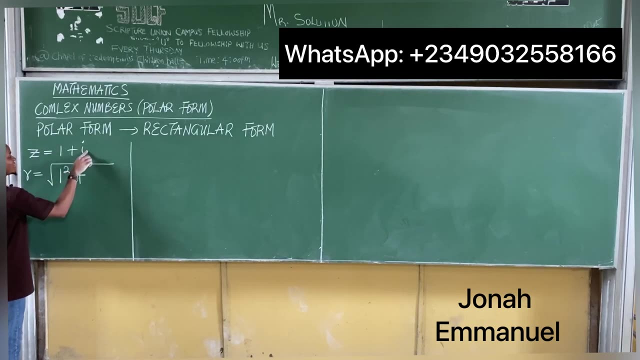 amplitude or the argument of this complex number. So first things first, let's find the modulus or the magnitude of this complex number. So we said the modulus or the magnitude r is simply equal to the square root of what I have here, 1 squared plus the imaginary part coefficient here. 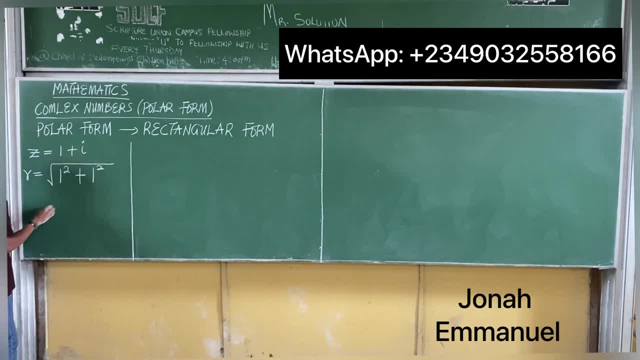 is 1 squared. So we did this in our previous class and we said: r is equal to the square root of 1 squared is 1 plus 1 squared is 1, that's equal to the square root of 2.. So I have root 2 as my modulus. 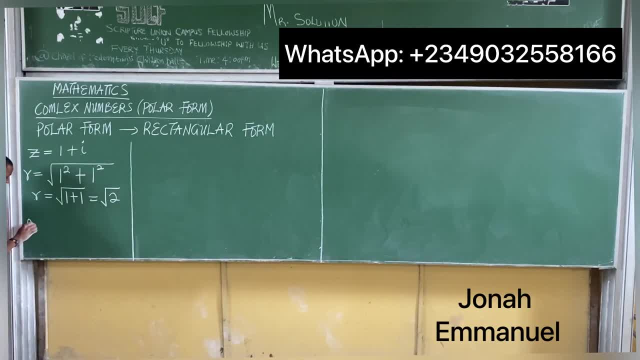 or my amplitude. Next up, we said theta as my modulus or my magnitude. So we said theta, which is the argument or amplitude, is equal to tan inverse of b, that's coefficient here, which is 1, all over the number I have here, which is 1.. 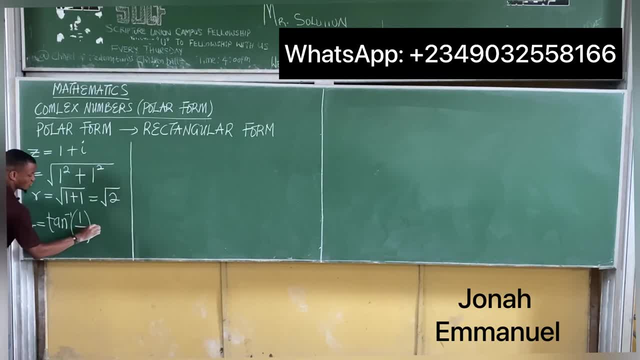 So we discussed this in our previous class- and that would be equal to 1 over 1 gives me 1, tan inverse of 1. let me punch that tan inverse of 1, the answer is 45. So I have 45 degrees. 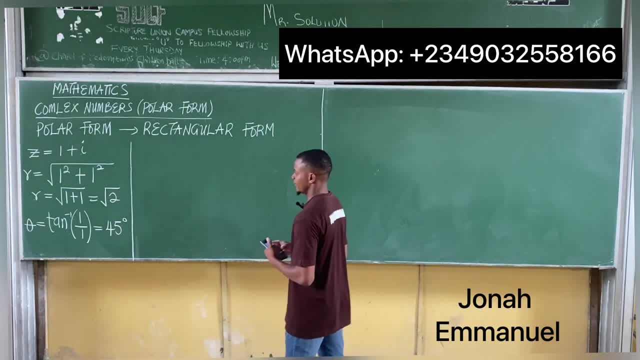 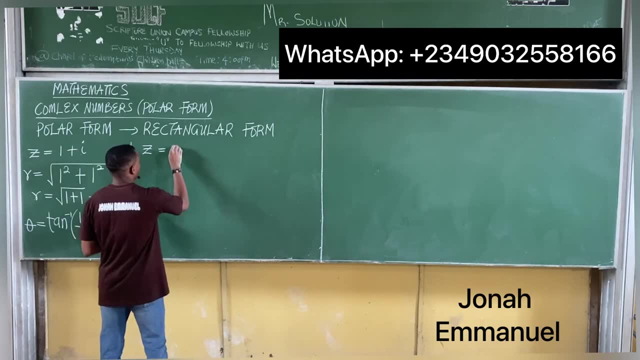 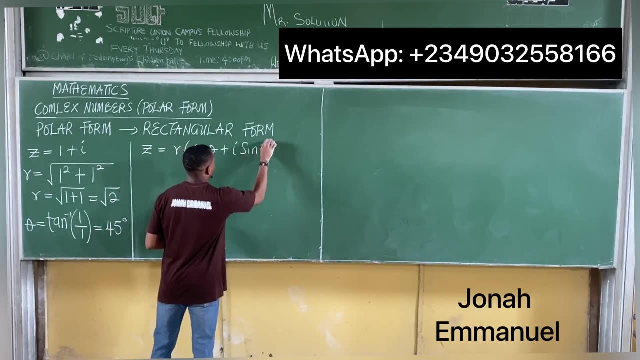 which is equal to 1 over 1.. So I had here a proved that this is the square root of 1 squared, plus the imaginary part coefficient here which I have here, which is 1 over 1.. And then I have here a proved that this is the square root of 2 squared. 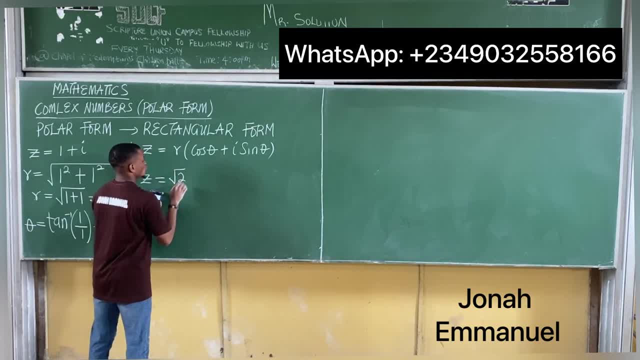 plus 1 over 1, which is 1 over 1.. This is 1 over 1, is equal to 1 over 2.. So this is 1 over 1.. cos we got theta here as 45 degrees, so 45 degrees plus i sine. 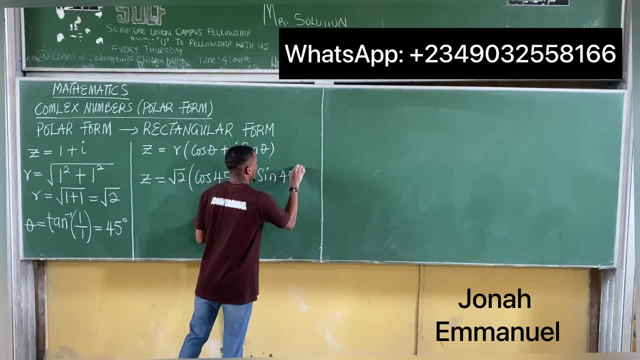 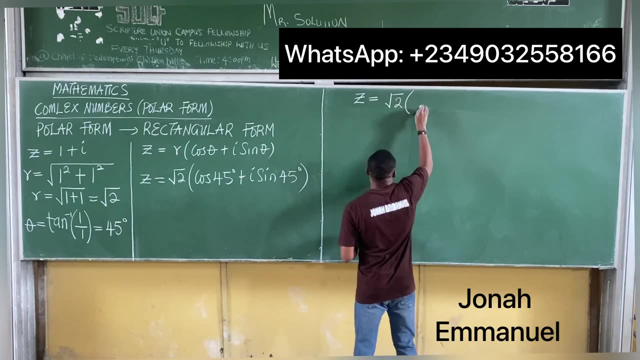 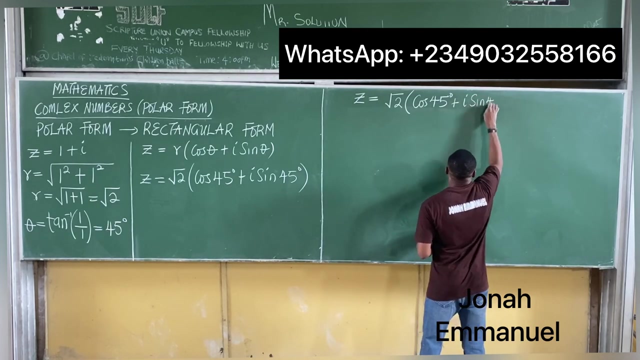 theta, which we said is 45 degrees. So this becomes the polar form representation of this complex number. So what if I was given the complex number z being equal to root 2, into cos 45 degrees plus i sine 45 degrees? This is in polar form and I was 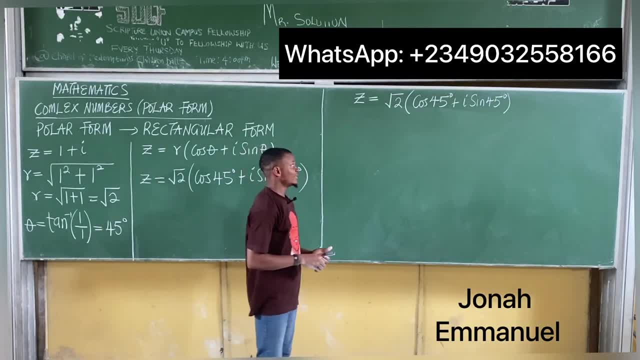 asked to convert it back to the rectangular form. What do I do Now? the idea is simple. The concept would be express this once: first in either decimals or sword or whatever. Just find the value of this and this, Then use the magnitude or the modulus to multiply it through. So it means that z will be equal. 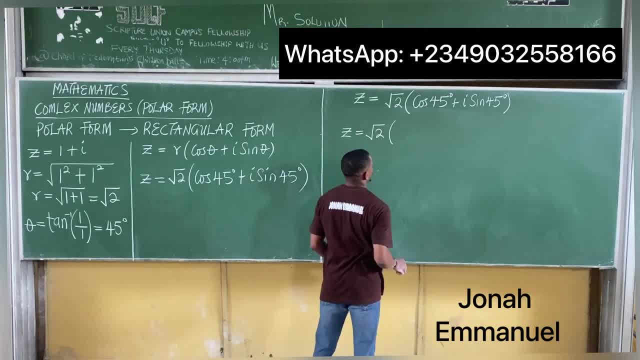 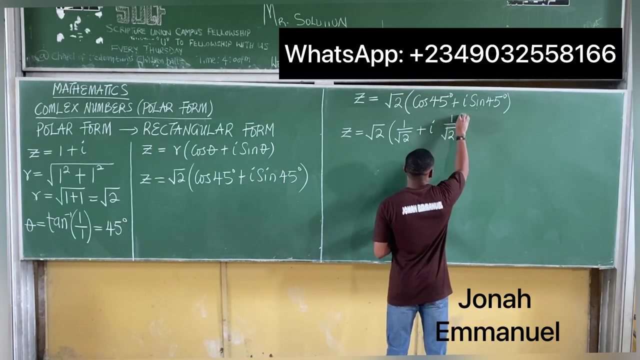 to square root of 2. into cos 45. If I punch cos 45, my answer is 1 all over root 2, plus i sine 45, the value is 1 over root 2 also, So 1 all over root 2.. So put this in: 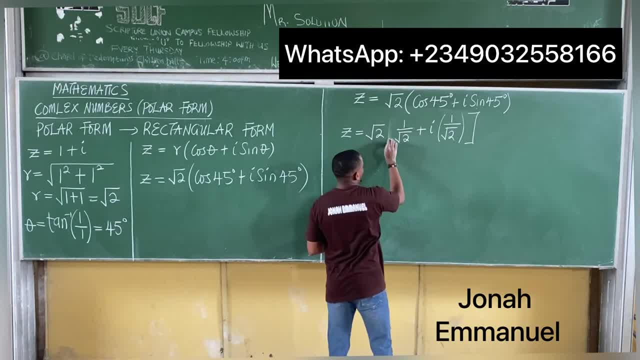 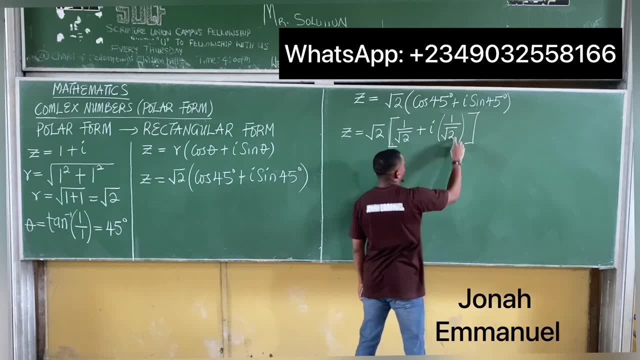 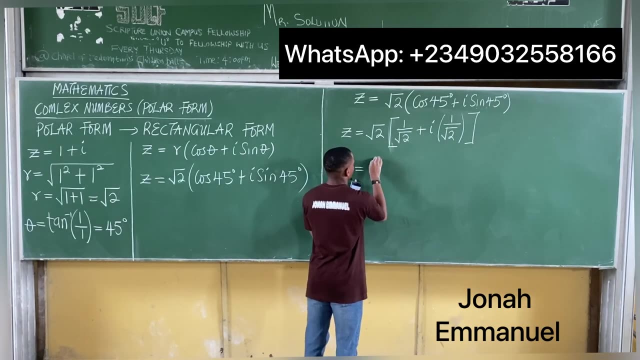 round bracket. change this to square bracket and then this: Alright. So cos 45 gives me 1 over root 2.. Sine 45 gives me 1 over root 2.. So if I multiply this, it means that z will be equal. to use this. to multiply this, it becomes root 2. 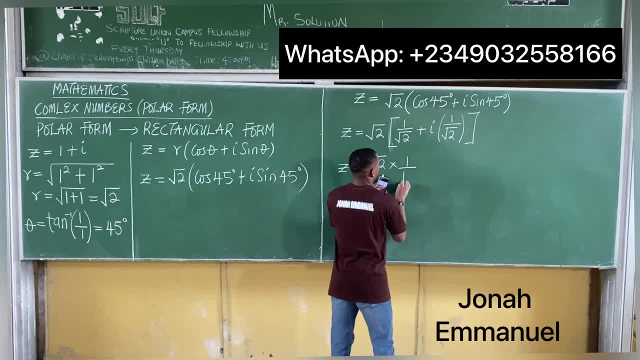 multiplying this one here: 1, all over root 2 times. use this to multiply this, but first of all have your i, So it becomes i. Use this one here to multiply this. It becomes root 2.. So dot root 2. 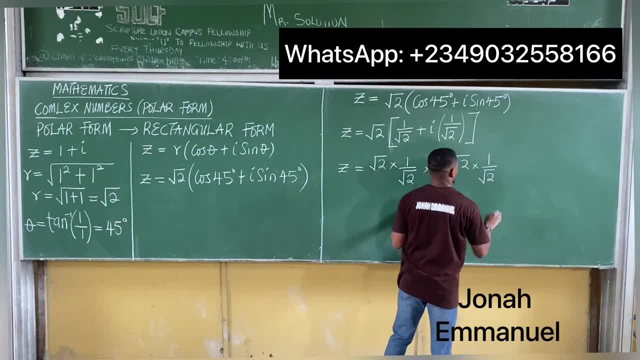 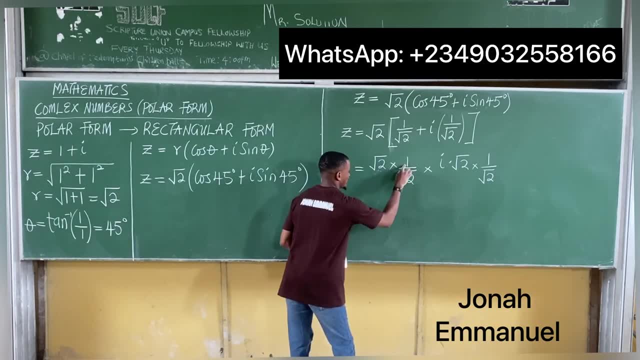 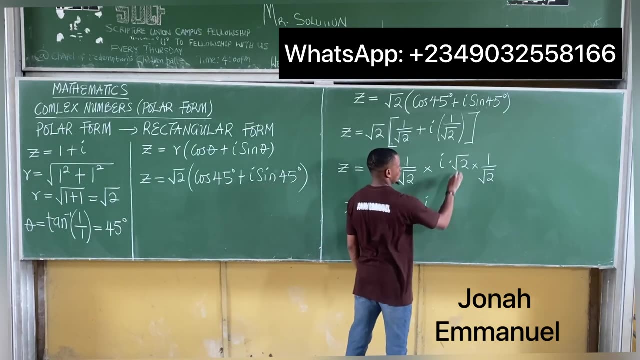 times 1.. 1 all over root 2.. So I have this answer. So hence z will be equal to. of course this becomes root 2. root 2 times 1 is root 2 over root 2 plus i into root 2 times 1 is root 2 all over. 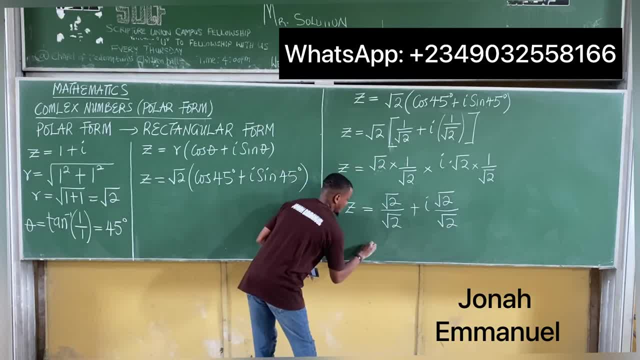 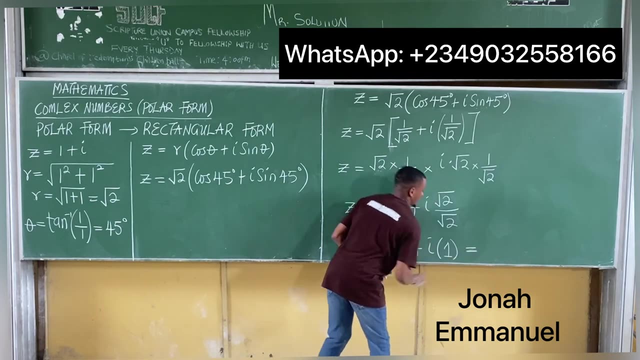 root 2.. From here it means that z is equal to root 2. divided by root 2 gives you 1 plus i. into root 2. divided by root 2 gives you 1.. So into 1. multiply this: It means that z is equal to I have 1, so becomes: 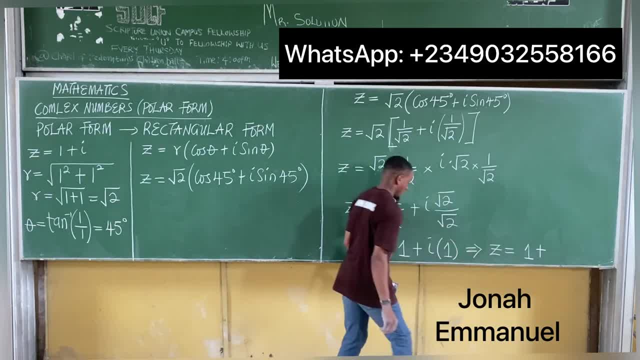 1 plus i times 1 is i, so z equals 1.. So z equals 1 plus i. That's exactly what we had from here, z being equal to 1 plus i of that. So that's what we have. So i plus i. da da dee. Do we follow through or not? 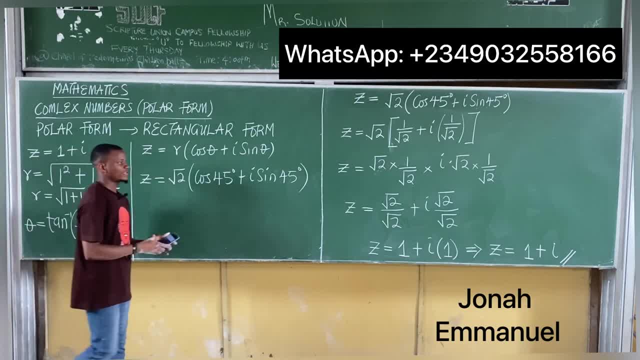 i is equal to i combined with i, So z is equal to 1 plus i. that's exactly we had from here that z in equal, equal to 1 plus i. Alright, so this is how you convert from rectangular form to polar form and from polar form back to. 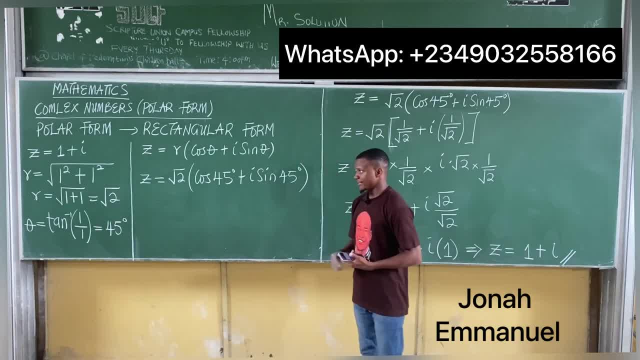 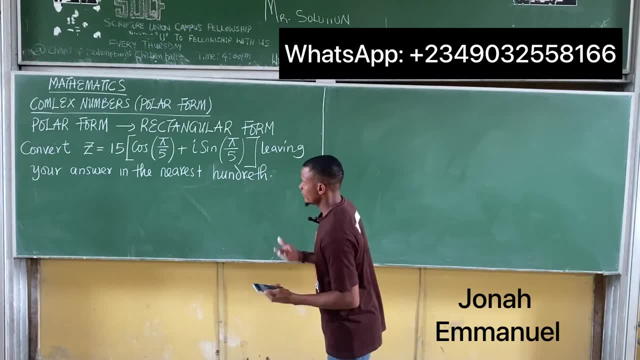 rectangular form. Alright, so this is how you do this. We'll take one more example on this and we're done with today's class. Alright, so let's look at the final example on how to convert complex numbers from polar form to rectangular form. In this case, we'll be considering 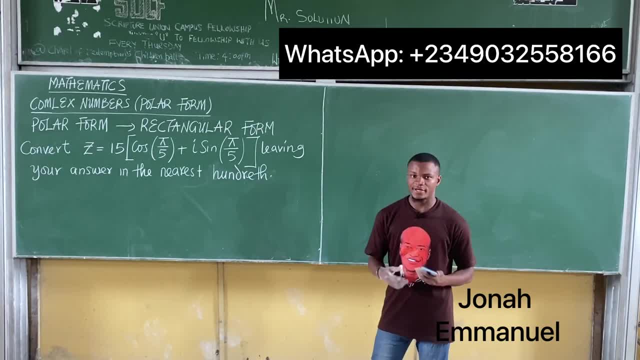 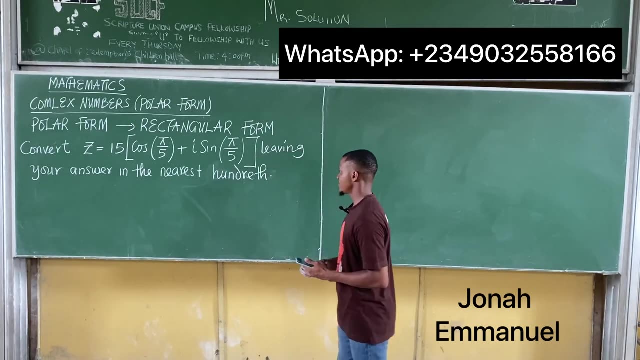 the polar form in radiance mode or in radiance form. So we have convert z being equal to 15, cos pi over 5 plus i sine pi over 5, to rectangular form- That's missing here- So to rectangular form, leaving your answer in the nearest hundredth. 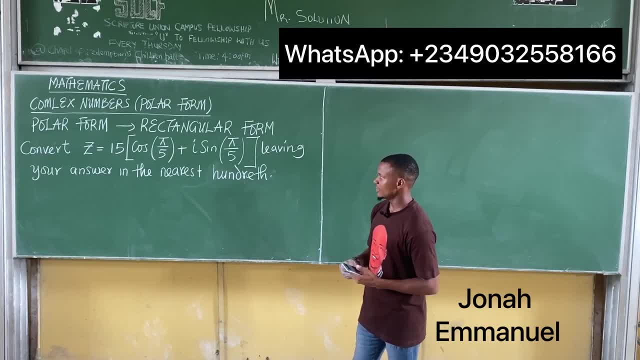 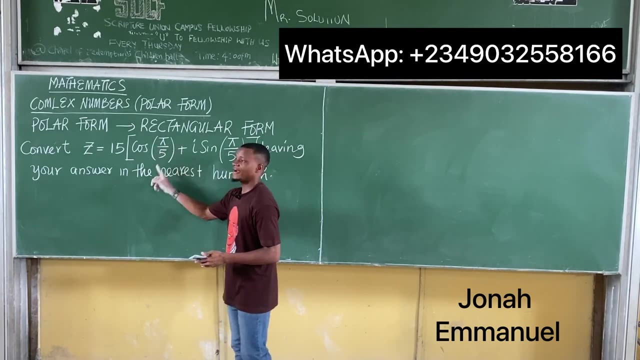 Alright, so let's get this done. How do you convert this one here to rectangular form, leaving your answer in the nearest hundredth? That would be easy. So your first task would be: if you know how to work with your calculator, your task would be: you can directly punch cos pi over 5. 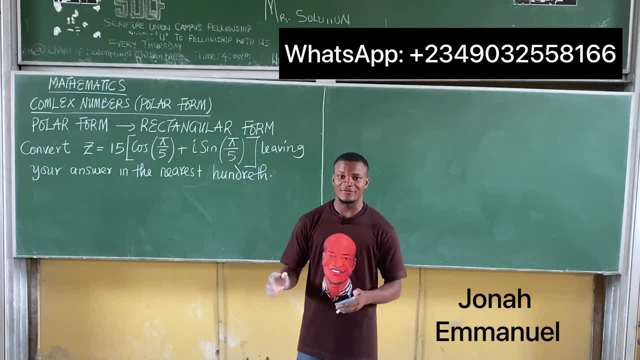 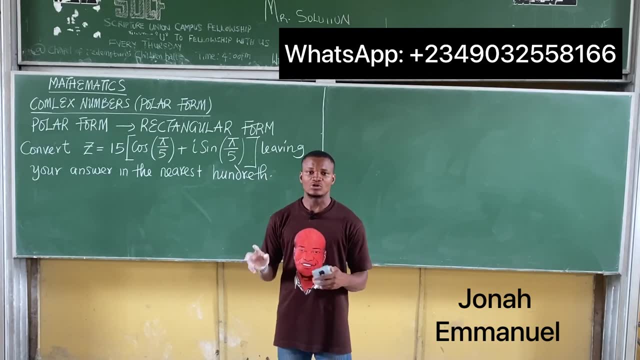 with your calculator. You'll have your answer directly, That's if you can convert the calculator from degrees to radians. So you should know how to do that. I will show you how to do the conversion from degrees to radians in our calculator hack class. Alright, so just simply check the description of this video. 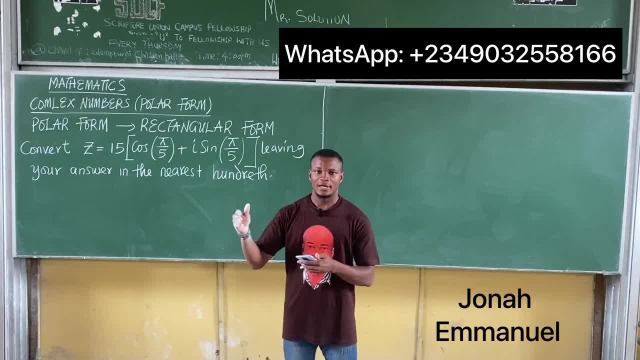 and you'll see how to punch your calculator from, or to convert your calculator from degrees to radians. So you can punch this directly. But then let's go back to this. So let's say we cannot do that, Alright, so what do we do? So let's first of all convert to what 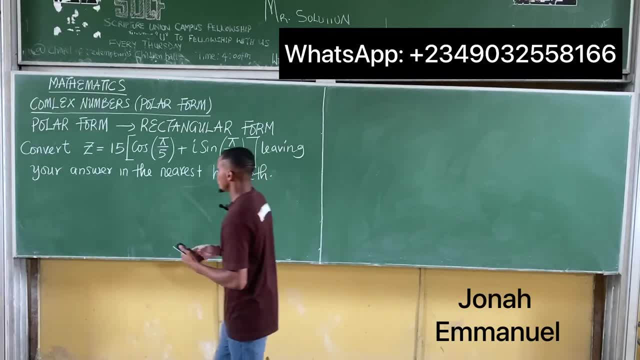 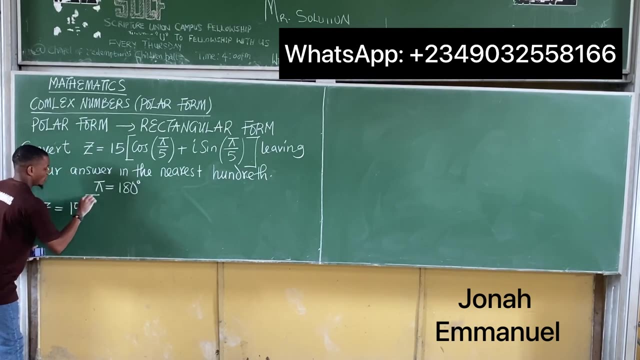 the degree form before we solve this. So first of all, convert this to degrees. We know that pi is equal to 180 degrees, So my task would be this. It means that z would be equal to 15.. Into cos, So, cos, pi. 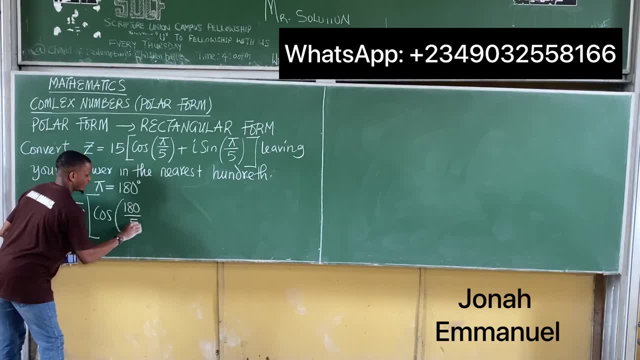 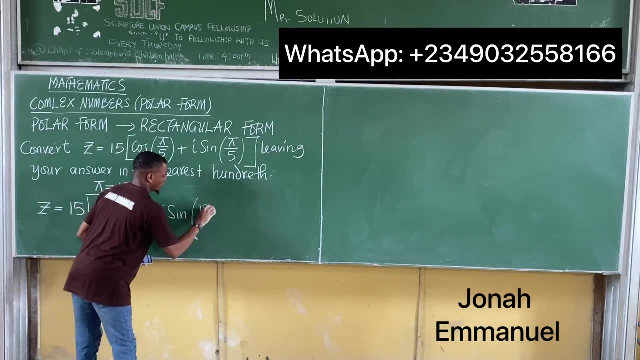 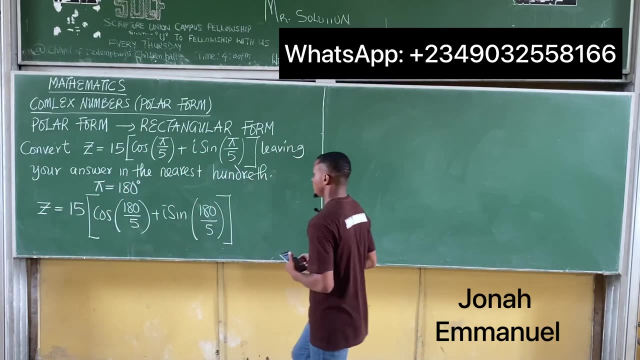 is 180.. So 180 all over 5, plus i sine 180 over 5.. So I have 180 all over 5.. So I have this one here, Alright. so from this it means that z is equal to 15 into. 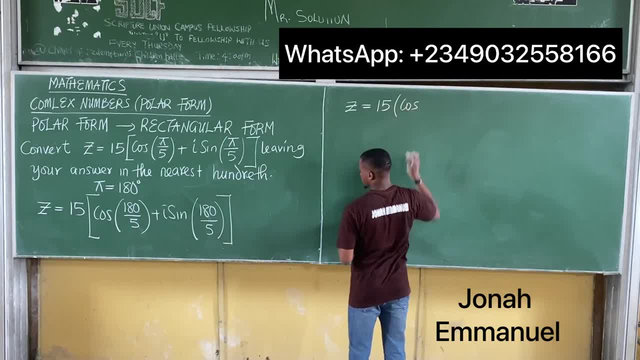 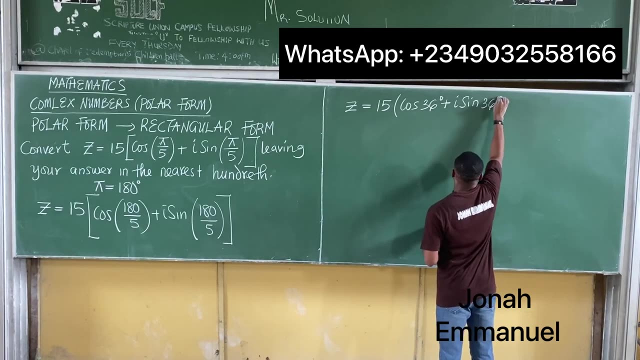 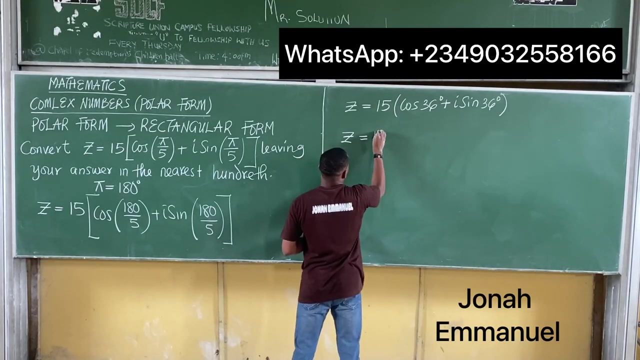 z cos 180 over 5, that's 36 degrees plus i sine. 180 over 5 gives you 36 degrees. So we have this one here. So from this it means that z will be equal to 15.. I'll simply punch: 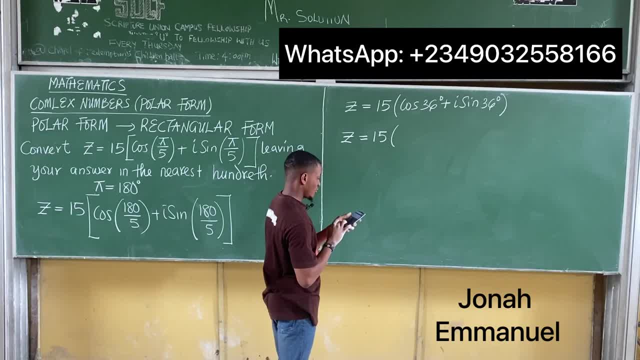 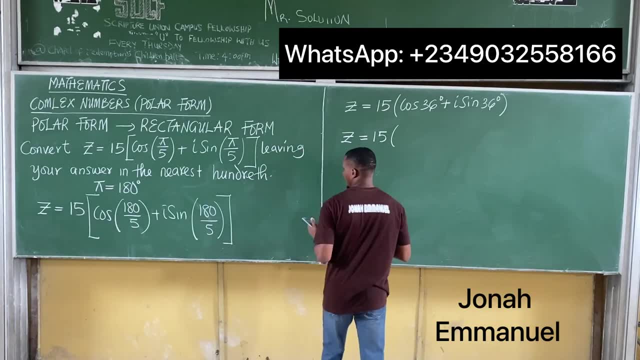 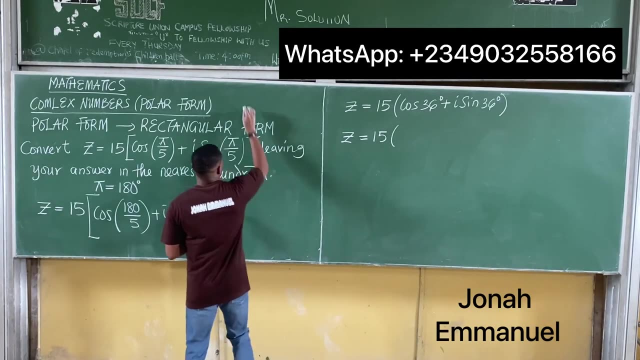 cos 36.. So, cos 36., cos 36.. That's about they said: your final should be in the nearest hundred. By hundred we mean two decimal places, Because in decimal places, let's say, we have a, b, dot, c. 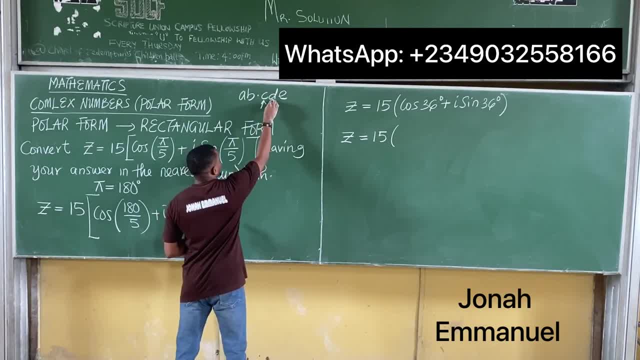 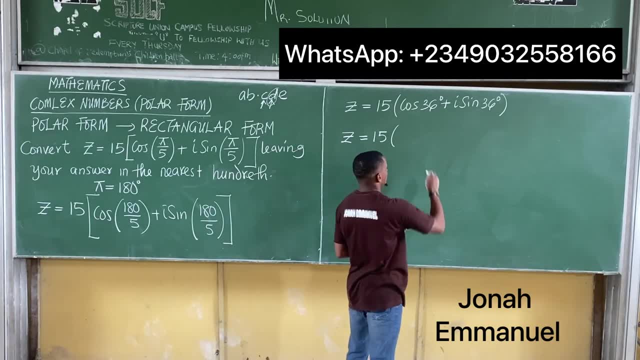 d, e. This is your nearest tenth, nearest hundred. So when we say nearest hundred it's simply two decimal places. For this one, I'll advise that you punch this one first in four decimal places, So cos 36 in four decimal places becomes. 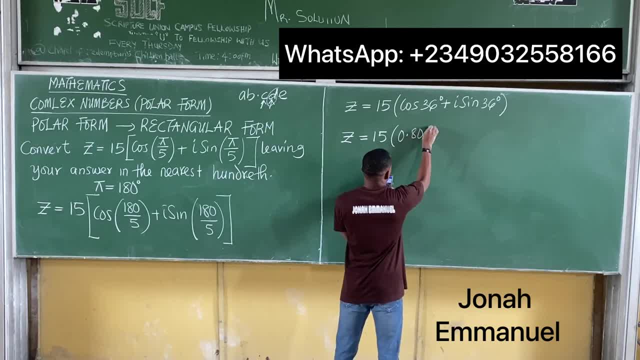 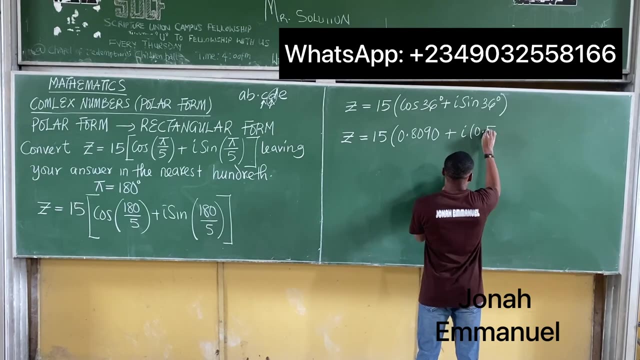 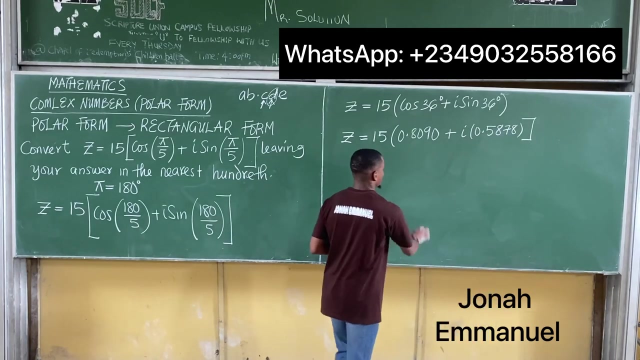 0.8090 in four decimal places, plus i into sine 36.. Sine 36 is about 0.5878 in four decimal places, So perhaps change this to square bracket. So I have this. So that's equal to my final answer. I can now multiply this by 15..